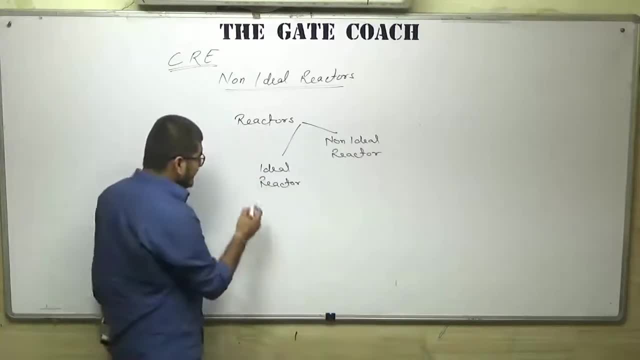 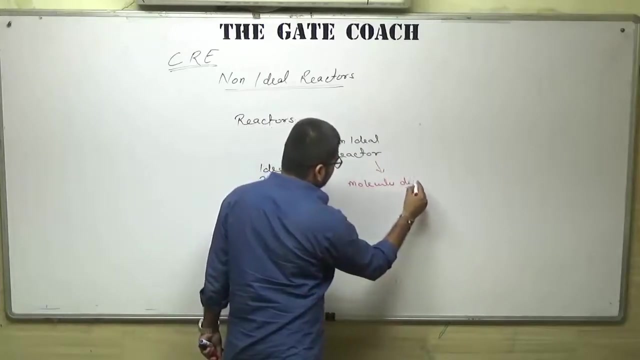 those. if I say in simple terms, ideal reactors are those where all molecules have same residence time. What is non-ideal reactor? What is ideal reactor? What is non-ideal reactor? What is non-ideal reactor And non-ideal reactors are those where molecules have different residence time. 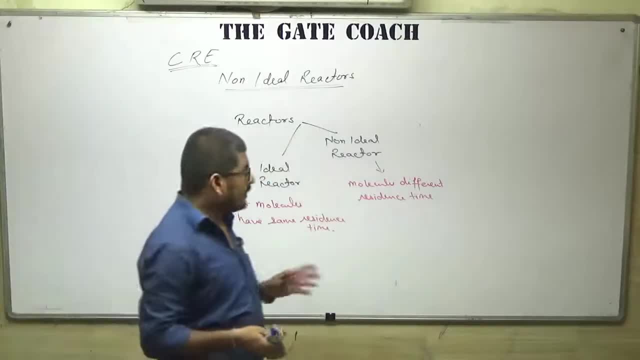 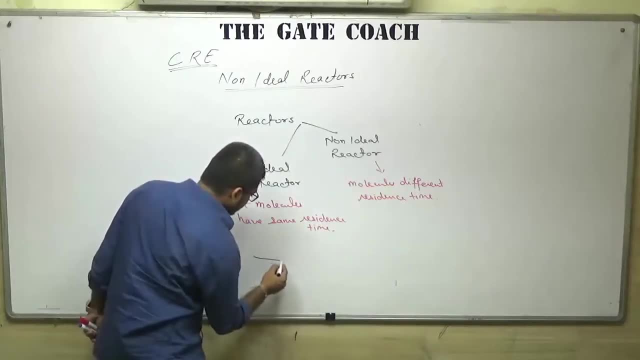 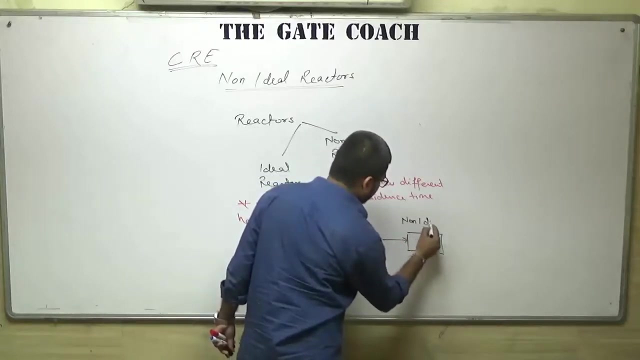 Okay, So what is the meaning of this term? So see, if I draw an ideal reactor, let us say this is a block diagram of any output ideal reactor and this is a block diagram for a non-ideal reactor. Molecules are going. 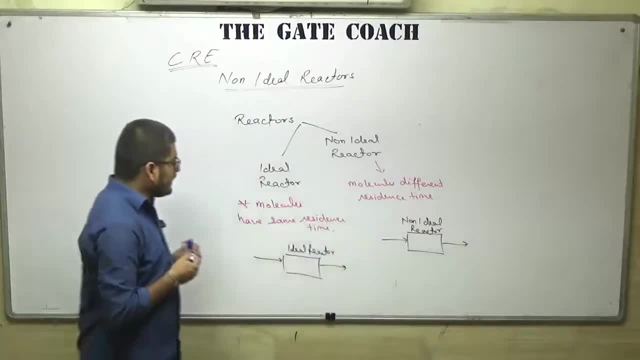 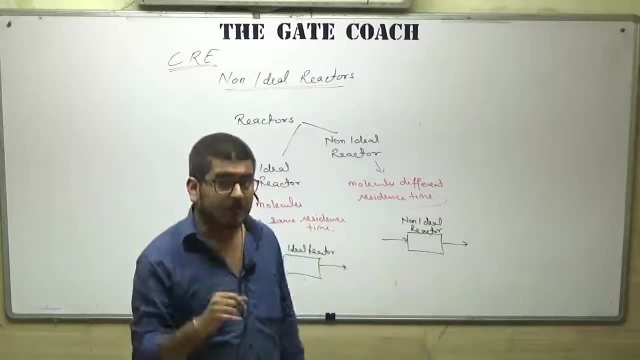 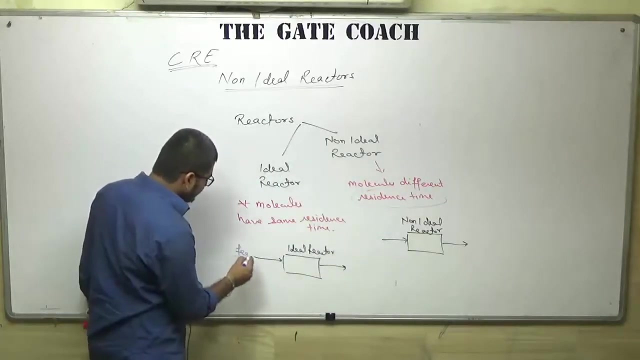 in leaving, going in and leaving- And what is the residence time? So all of us know that residence time is the time spent by a molecule within the reactor. So in case of ideal reactor we know that molecules are going in with some bulk velocity. let us say that is U0 and the 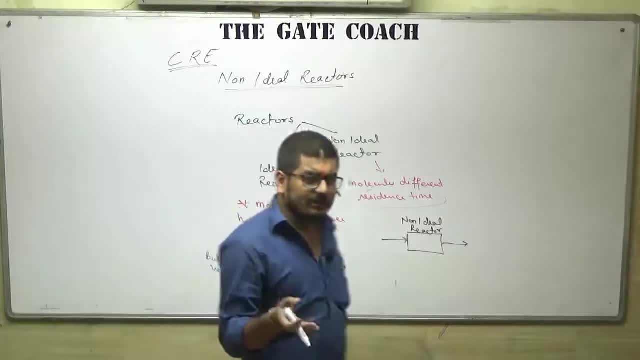 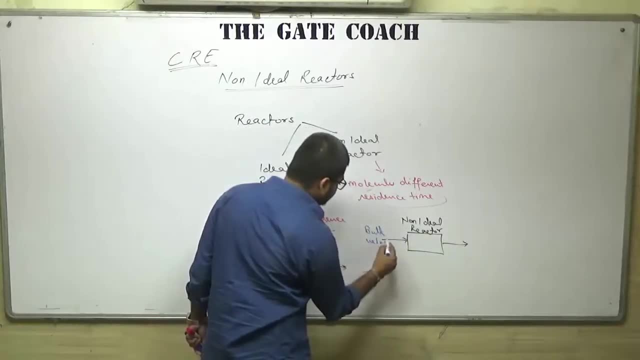 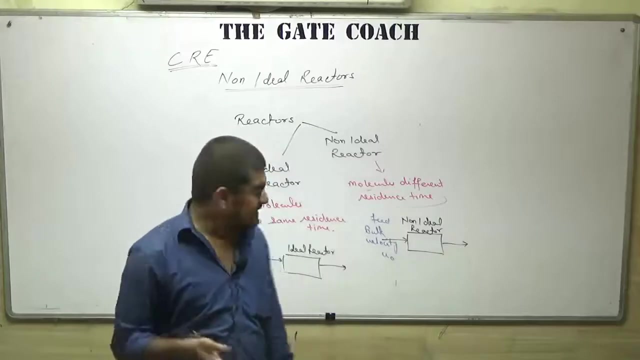 bulk velocity of all the molecules will be approximately same. In the same way, here, in non-ideal reactor, the bulk velocity of all the molecules will be approximately same. The bulk velocity of feed, let us say U0, and that is, that too- will be same for all the. 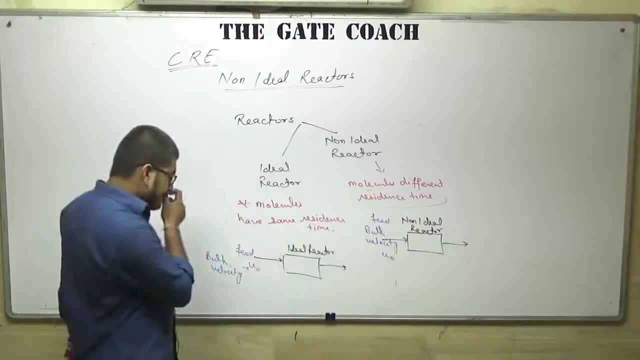 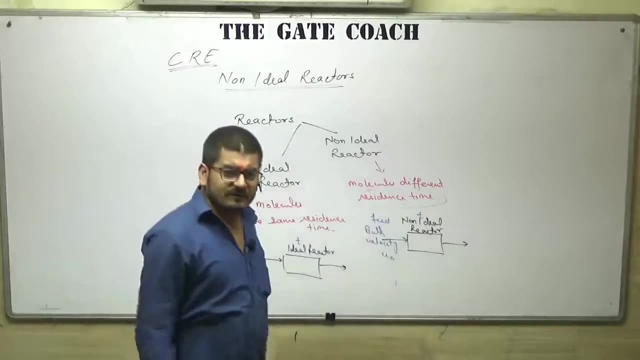 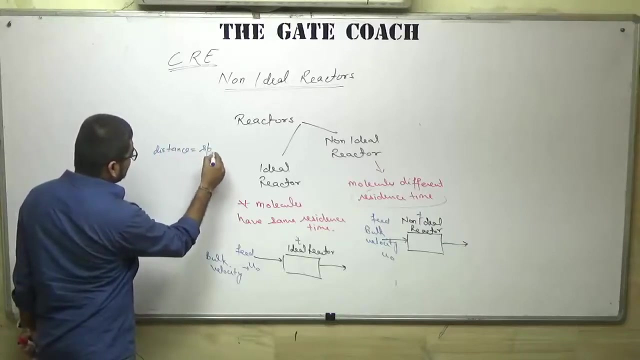 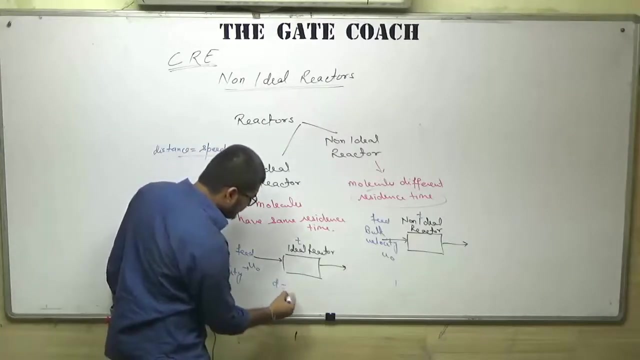 molecules approximately. okay, And this is the residence time T. So now all of us know that distance is equal to speed into time. So in the same way here, distance travelled by molecule within the reactor will be the product of the bulk velocity of molecule and multiplied by their residence time In the 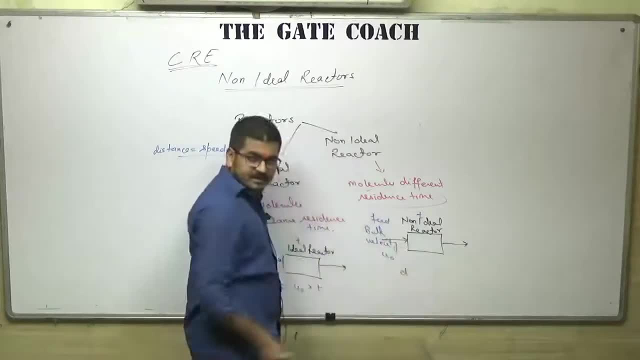 same way here. the distance travelled by the molecule within the reactor will be equal to the bulk velocity of molecule and the residence time of the molecules. So now you can see that in case of an ideal reactor, bulk velocity is saying U0, 2- fuckin maths. I hope you like our lecture and please do like us with your comments and also please subscribe our YouTube channel and again, do not forget to click on the bell icon and will be able to get product here also link in the description box. A quick know that after. 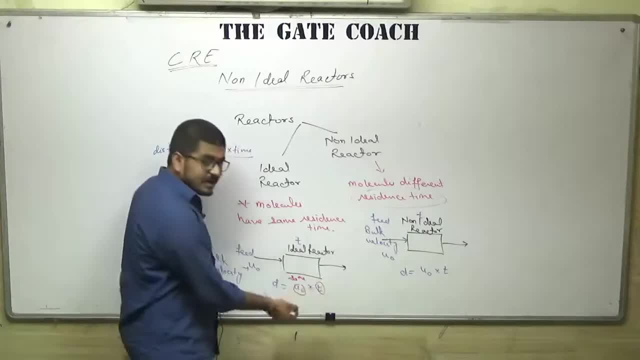 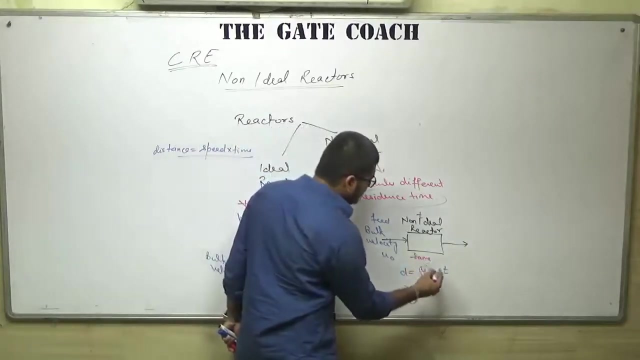 velocity is same and residence time is also same, So the distance travelled by all molecules will be same as well. Okay, But in case of non-ideal reactor, bulk velocity of all the molecules is same, but the residence time spent by the molecule within the reactor will be. 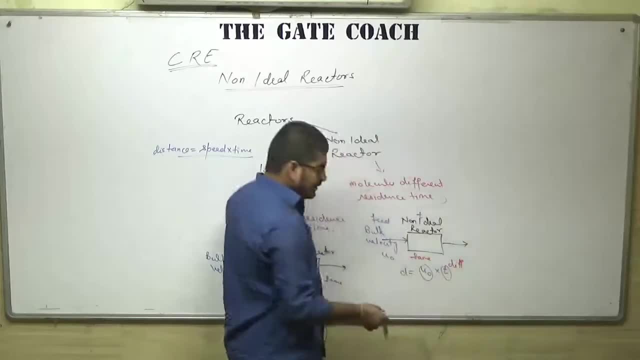 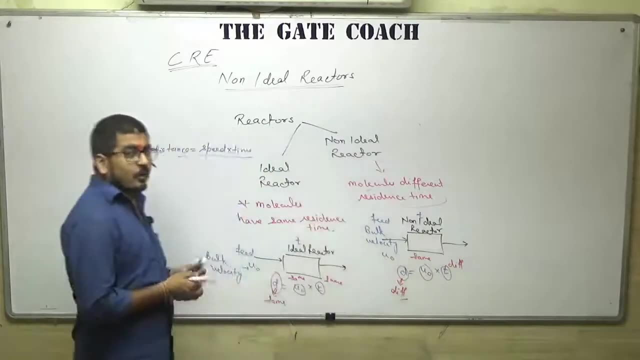 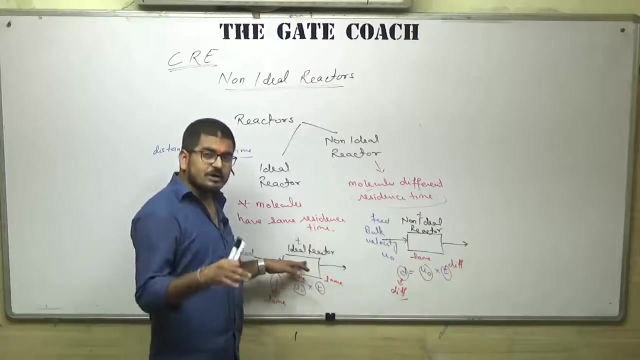 different. So the product means the distance travelled by the molecule will be different as well. So what is the meaning of that thing? If you see in a different way that in ideal reactor all molecules travelling the same distance, Okay, It means all molecules. 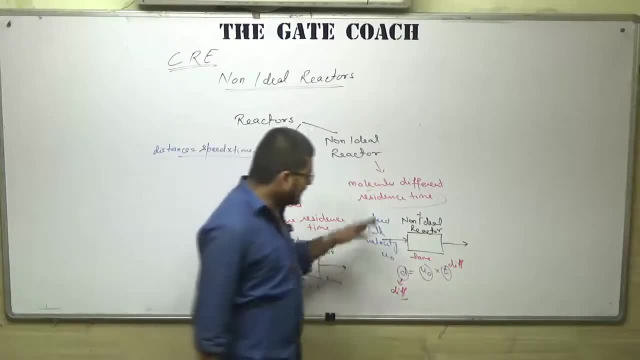 have same flow path but in case of non-ideal reactor distance travelled by all molecule is different. So it means we can say the flow path for all molecules is the same. So we can say all molecules travelling the same distance. molecules is different in case of non-ideal reactor and flow path is. 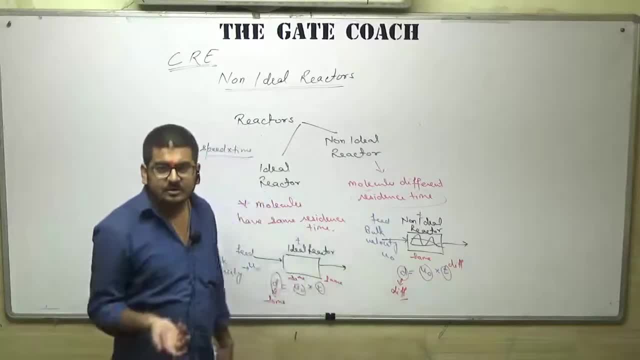 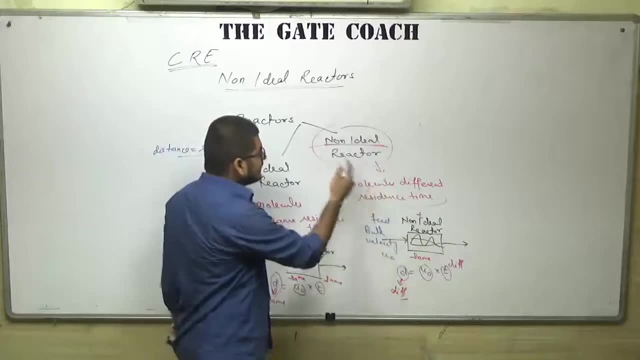 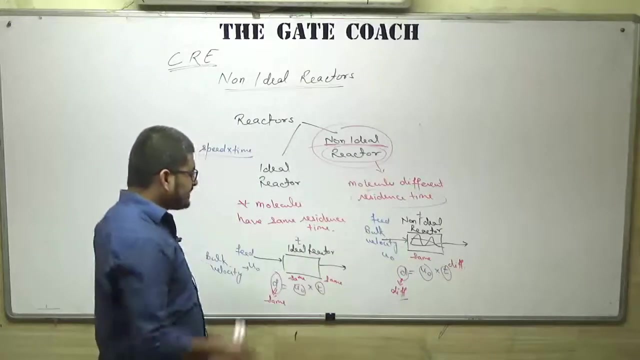 provided by the reactor. that depends on the reactor geometry. that's why we use the term non-ideal. reactor means this non-ideality is basically the characteristic of reactor, not the reaction mixture or anything else. okay, I think it is clear to all of you why the residence time in non-ideal reactor is. 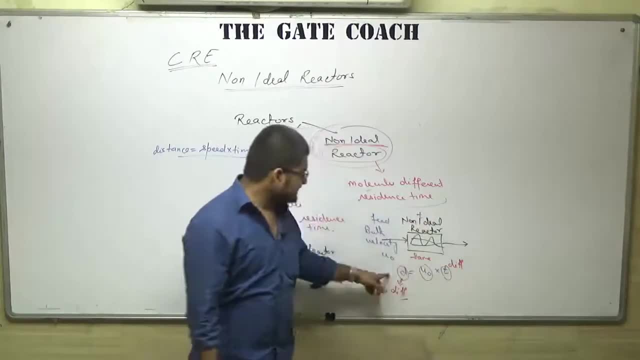 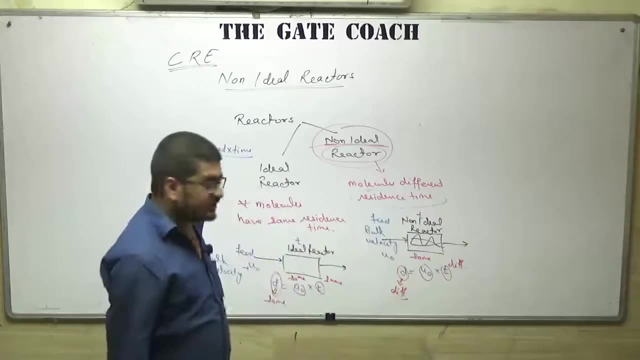 different for different molecules, because the distance traveled by molecules, the flow path of the molecules in the reactor is different and that depends on the reactor geometry. okay, so that is something about the non-ideality of reactor. now we will talk about the causes of non-ideality: why the molecules? 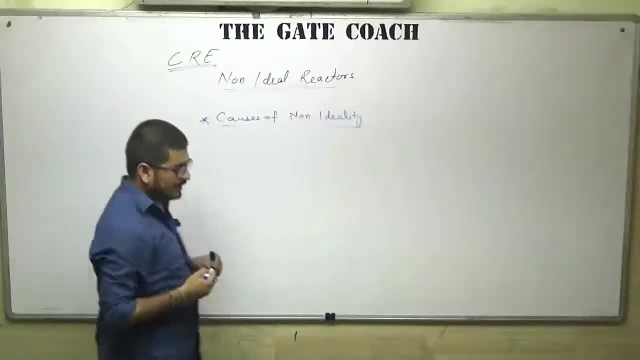 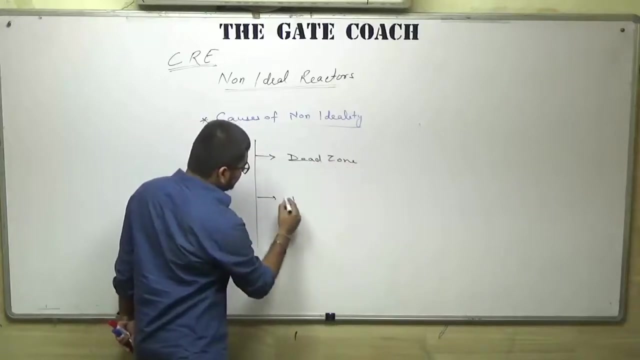 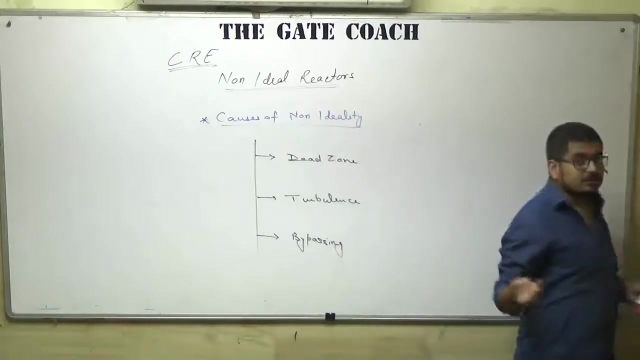 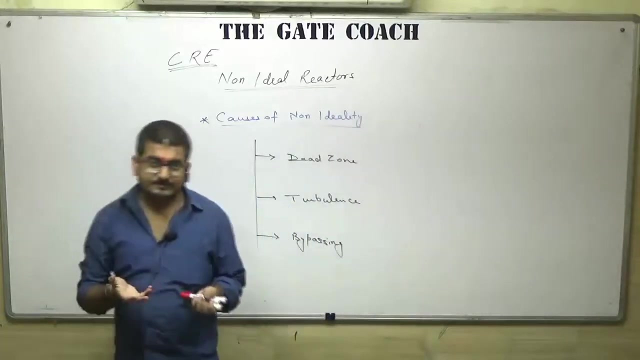 have different residence time here. so basically the there are n number of reasons and, yeah, non-identity, but here we will talk about mainly three. one is dead zone, second one is turbulence and third one is bypassing. okay, so what is that zone? as the name suggests, dead zone. so the probability of that person to come. 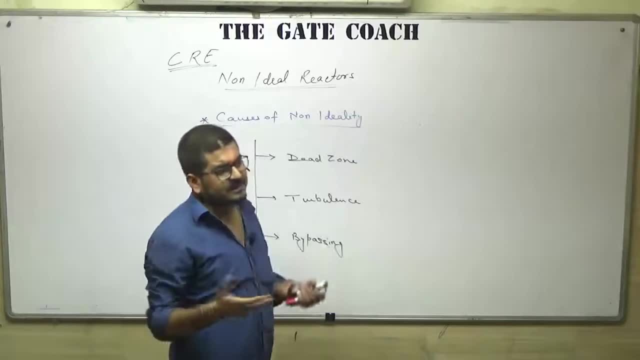 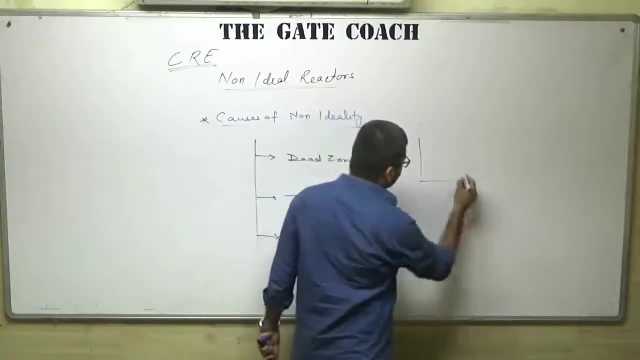 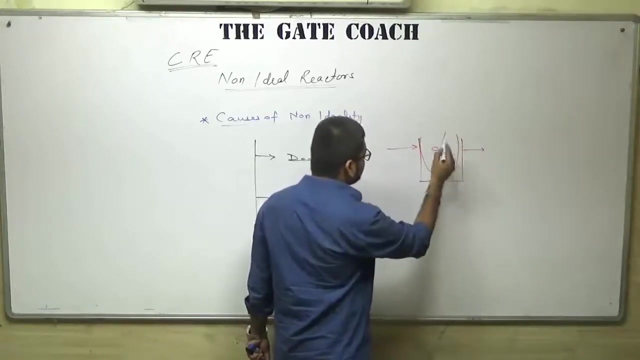 back in real life is almost zero, or we can say he may come back in real life after infinite time. so, in the same way, in a reactor where we have extreme corners, this is inlet, this is outlet, and we know that normally the mixing mixture profile is parabolic because 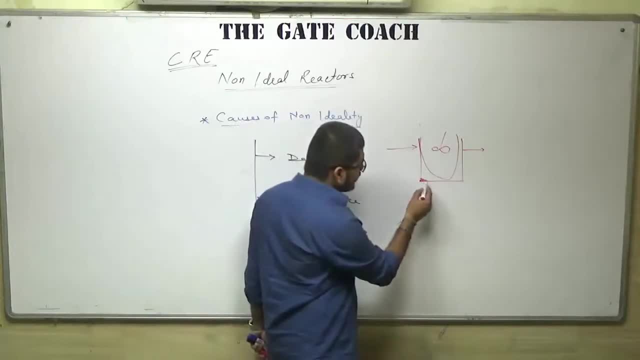 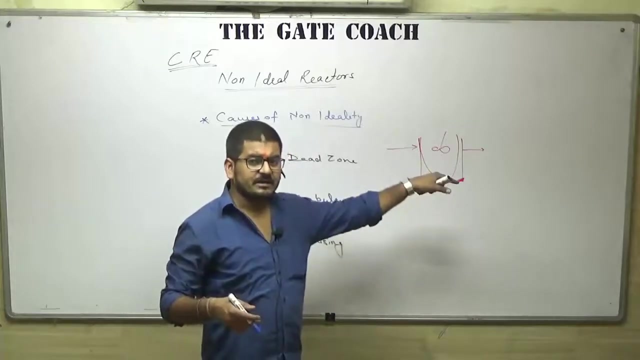 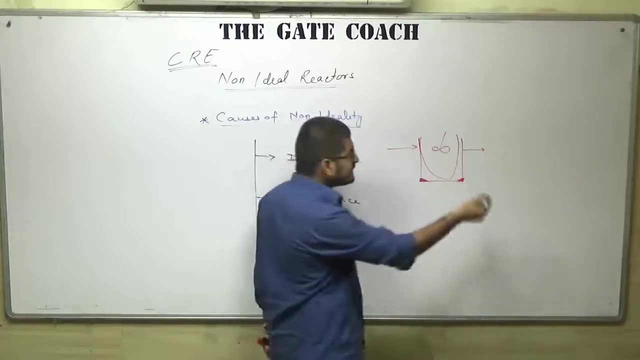 of the agitation. so, because of these extreme corners, if any molecule got trapped in these, then the probability of those molecules to leave the reactor will be almost zero, and thus time spent by these molecules when they are not leaving the reactor then obviously the time spent by the molecule in the 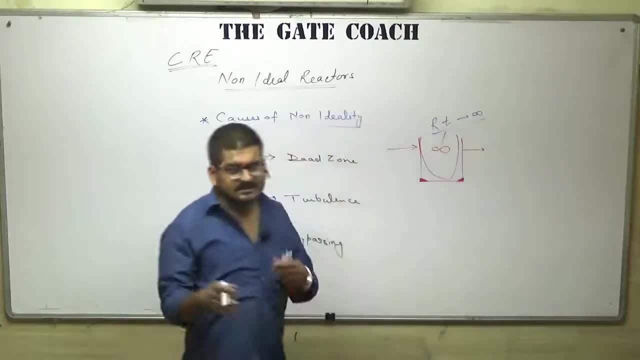 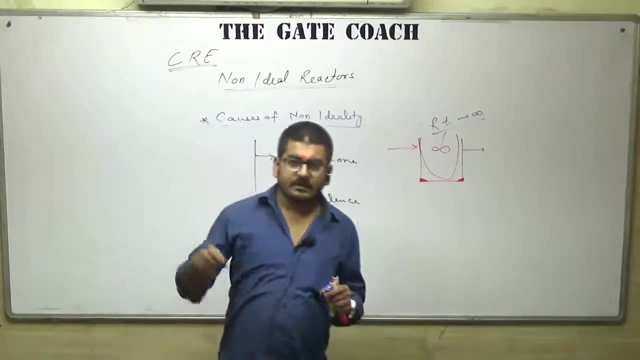 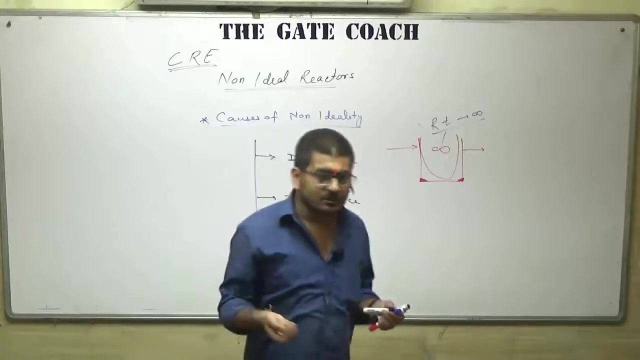 reactor, the residence time will be infinite. it is just like when we observe on a daily basis and we go to our house for cleaning. so if there is an extreme corner, you can try to clean it with the help of a brush or anything, any clothes, then no one will come. you get it. 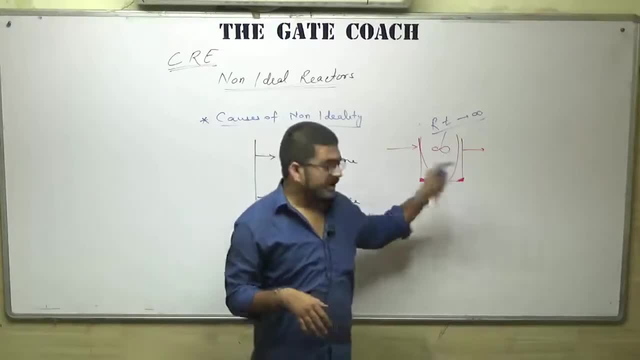 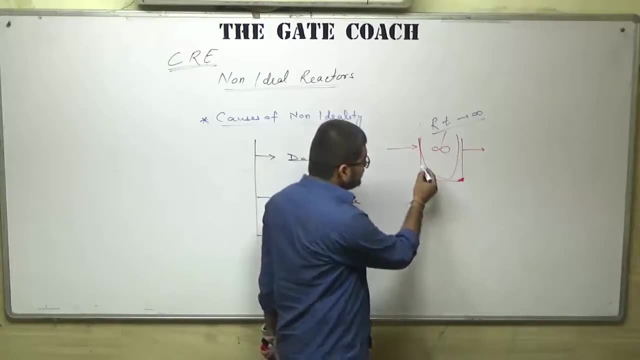 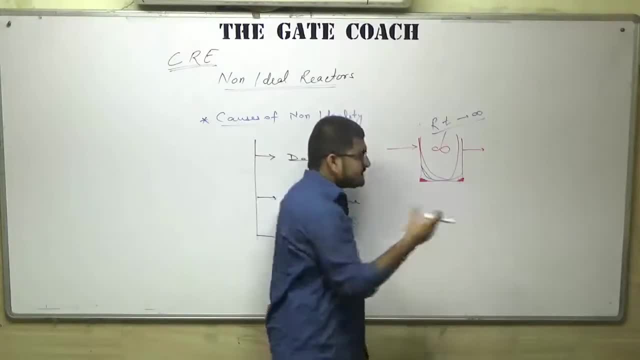 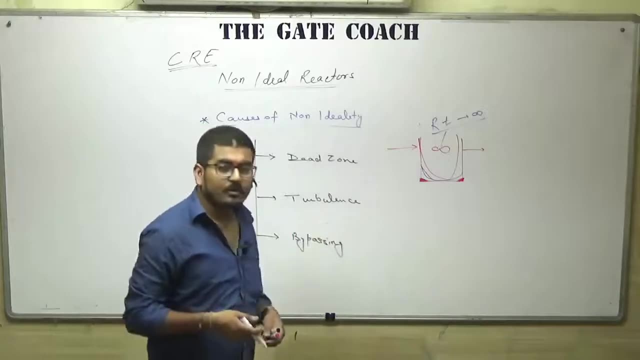 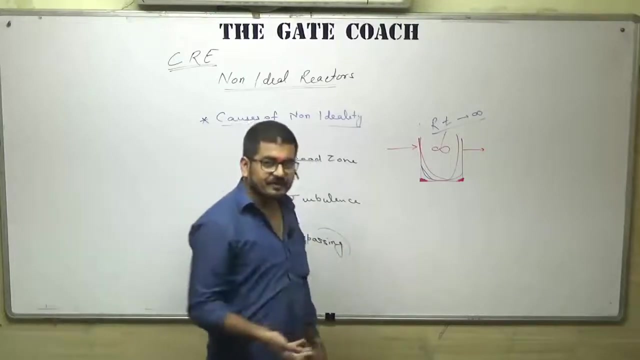 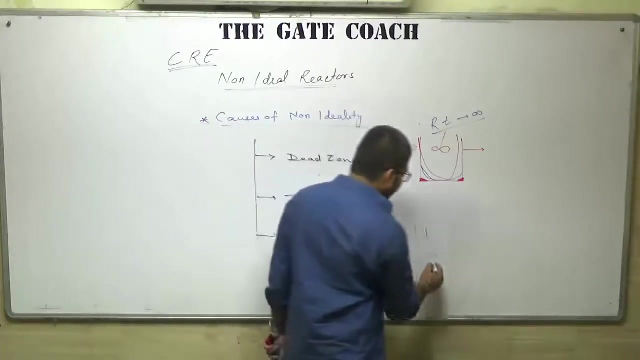 reactors have hemispherical or cylindrical bottom to avoid the extreme corners, so that we do not have the problem of dead zone. And next one is bypassing what is bypassing: to skip the process when some amount of inlet is directly sent to the outlet, by skipping the process in the same way, here in this reactor. 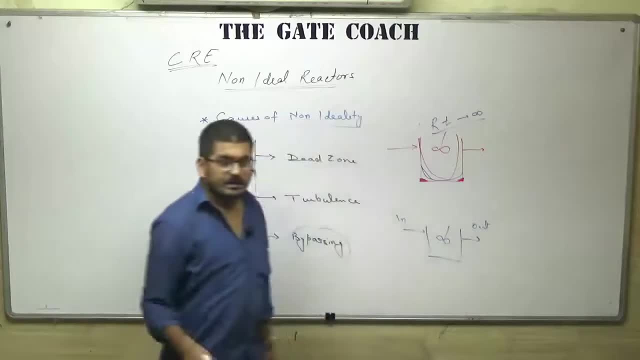 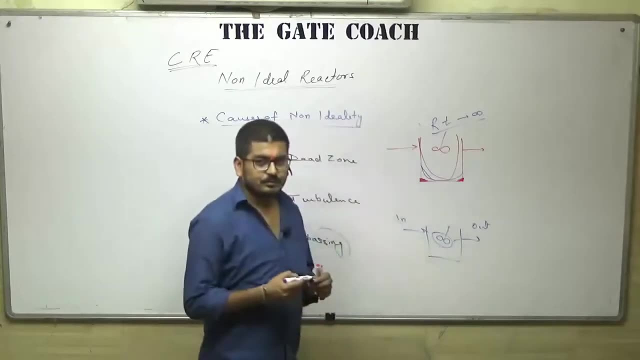 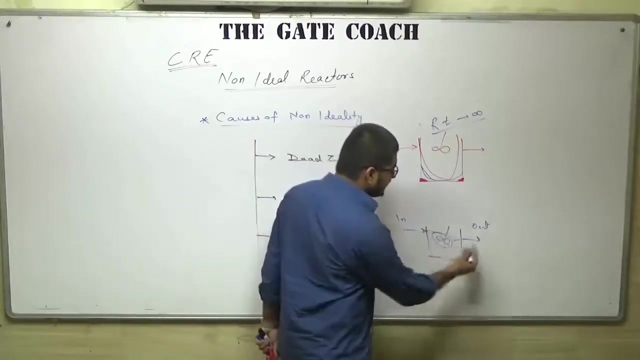 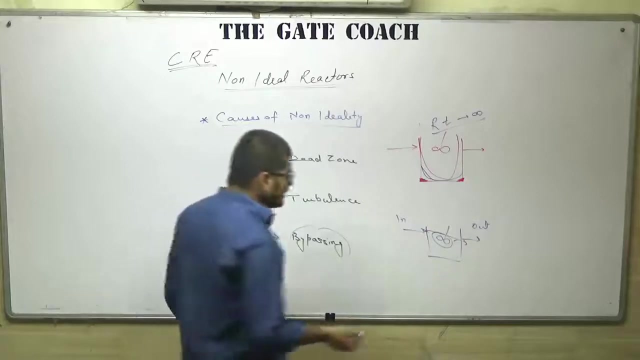 this is inlet, this is outlet. okay, logically, if the molecule is going in the reactor, it should get mixed and then leave. that is the path the molecule should follow. but what happened in practical life? there are some molecules which directly go to the outlet. either they have very high velocity or very high inertia force, so they directly move to the outlet. 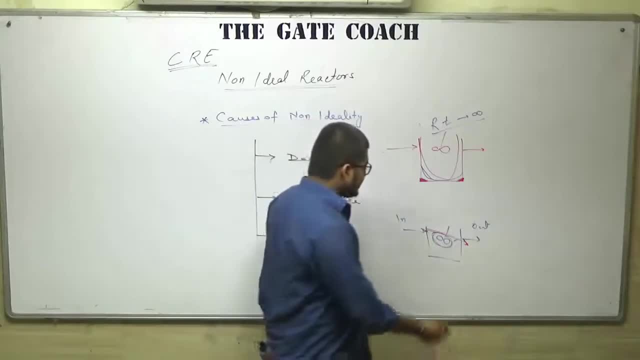 and skip this mixing zone. Okay, So we say that molecules are skipping the mixing, skipping this zone so means they are bypassing, and in this case you can see, the residence time of the molecule in this reactor is very small, means almost zero or short residence time, you can say. 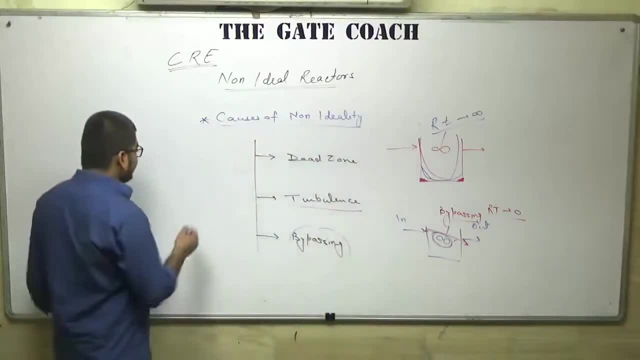 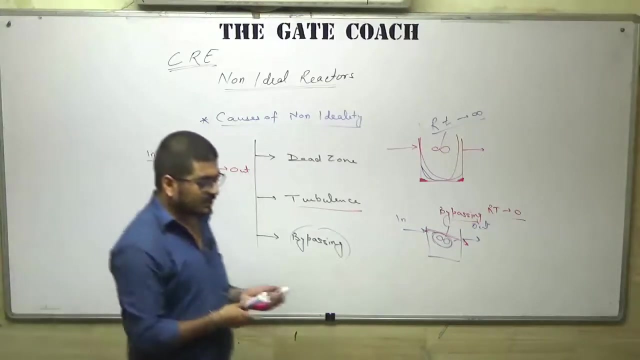 Next one is turbulence. what is turbulence? basically, it is related to mixing. This is inlet, this is outlet, this is agitator, and you know that there is a mixing zone. maybe you have heard about the term vortex formation and all okay, so you know that vortex formation, 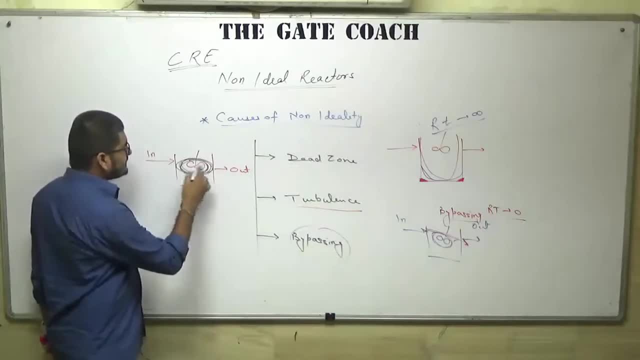 is what? that there are some molecules got trapped in the mixing zone. now, if a molecule gets trapped in a vortex, then it keeps rotating in it continuously, following the same path, and because of that, if there is any new molecule, then it should be kept in the mixing zone. 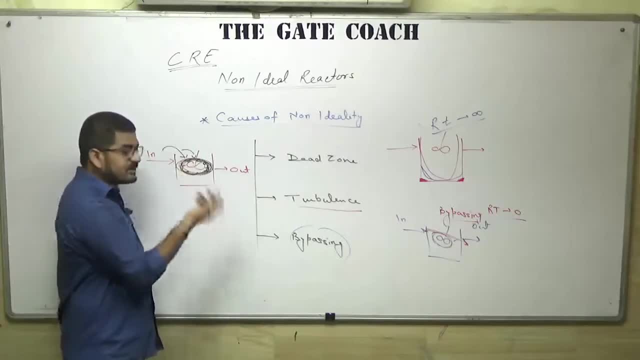 Okay. So we are done, Okay, Okay, We are done, Okay, We are done, Okay, Okay, Okay, Okay, Okay. molecule: it will not enter in the mixing zone because there is no vacant space and, in the same way, if any molecule is trapped in this, so it will take a very long time, very large. 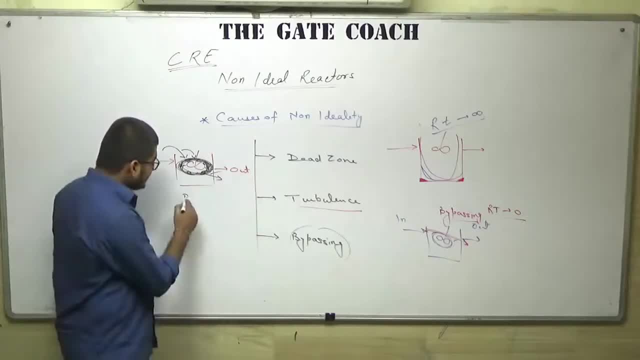 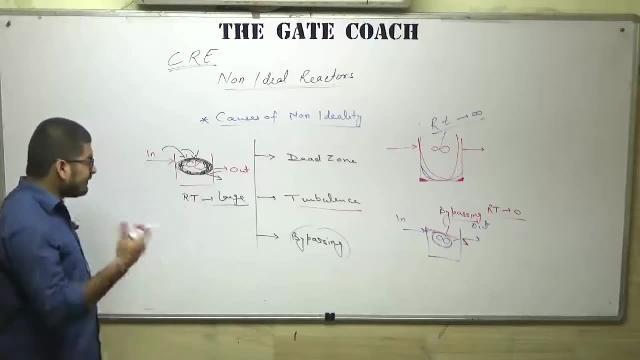 time to leave the reactor. okay. that's why in case of turbulence, the residence time is very large, not infinite, because it is a part of process. so it definitely the molecule will leave the reactor, but after very long time. so if you draw a curve between number of molecules, 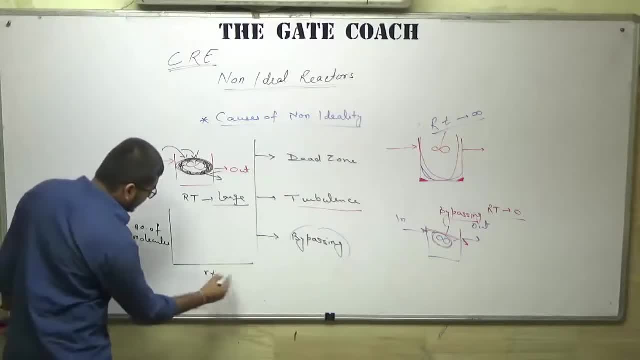 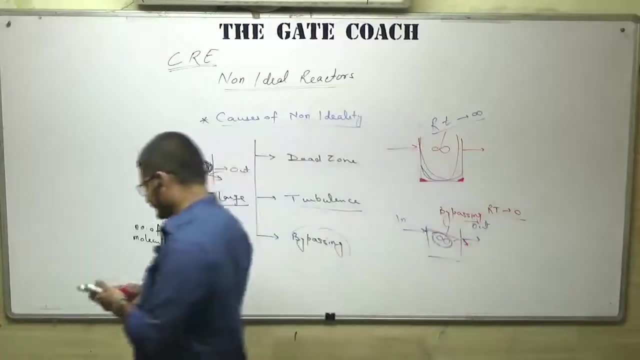 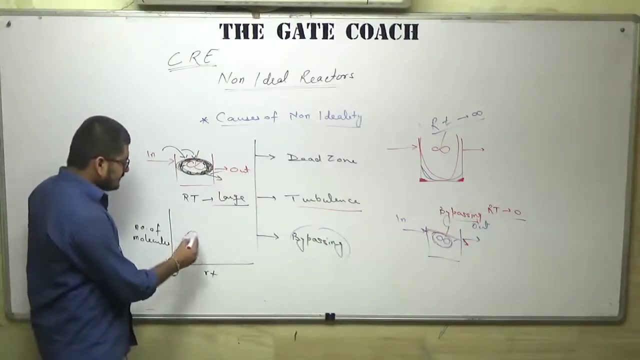 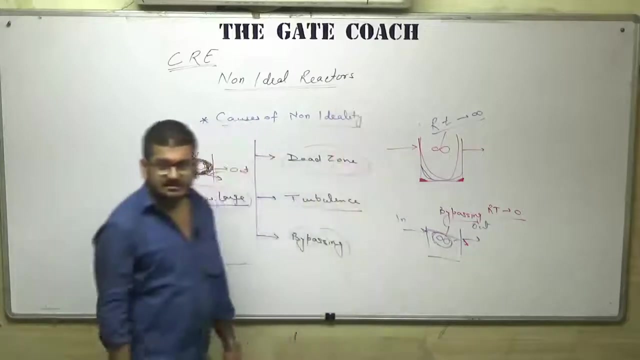 leaving the reactor to the residence time then, because of the bypassing, some molecules have very small residence time so they will leave early. then some molecule will leave near the mean residence time. Then some molecules will leave, because of turbulence, having have very large residence time. and if there is any molecule in that zone which has infinite residence time or 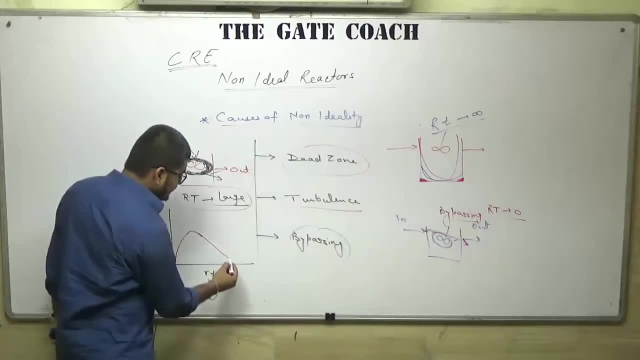 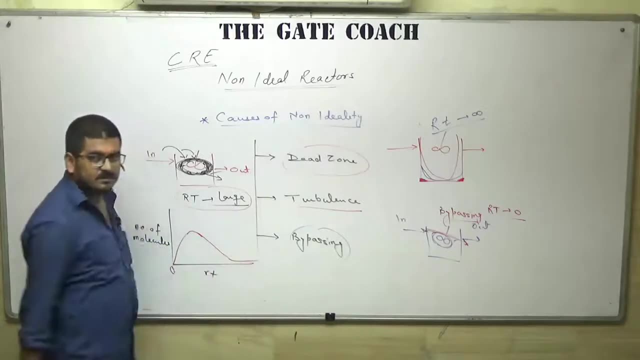 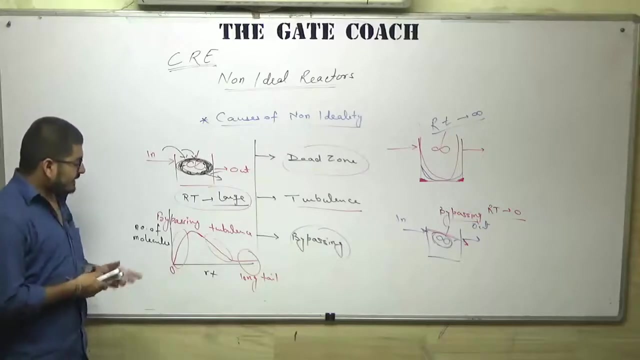 very, very large residence time, so that molecule will not leave the reactor. so that's why this curve will never going to touch the x-axis. okay, and this long tail represents the dead zone in the reactor. Okay, This is turbulence and this is bypassing. okay, very short residence time and we can. 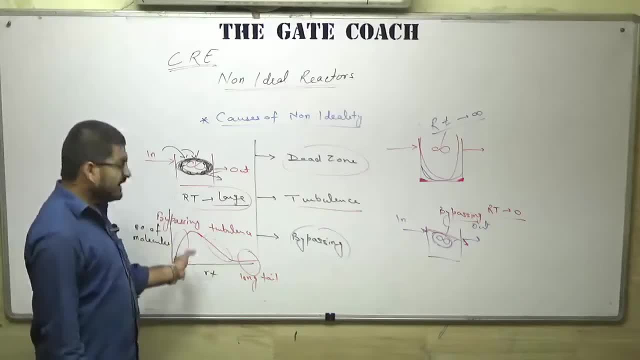 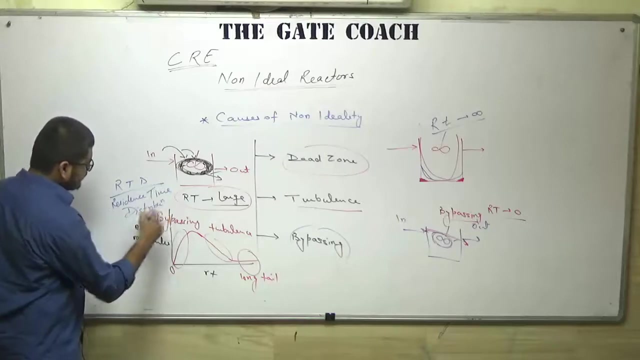 see that in non ideal reactor molecules have different residence time. so when we draw the curve it is like a distribution curve and the analysis of this distribution curve of residence time of different molecules is known as Residence RTD, that is, residence time distribution. okay, so this is something about basic part. 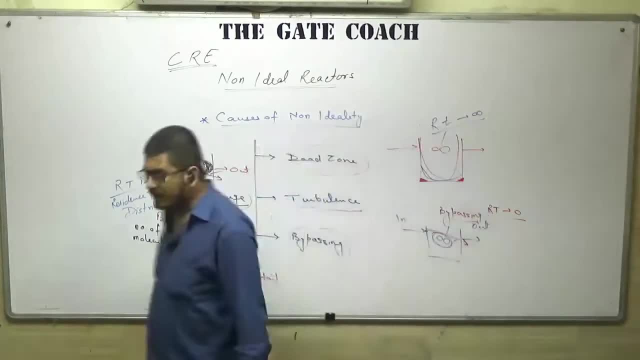 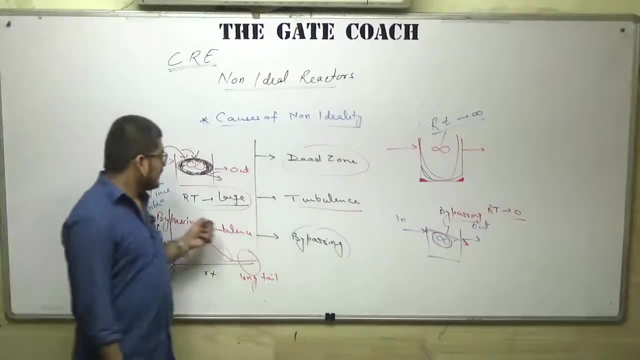 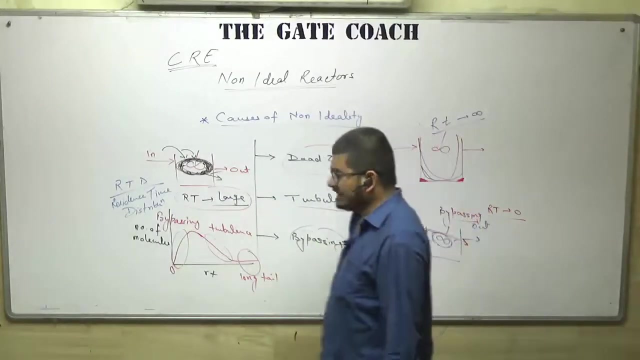 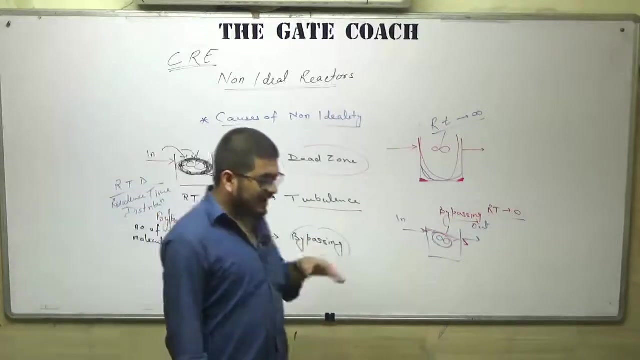 after that I will discuss about the how to find out the residence time distribution curve in the reactors and what is the parameter or what is the element we use to identify that residence time distribution curve- that is basically tracer- and how to inject that tracer in the reactor, but that I am not going to discuss in this video. that we will discuss. 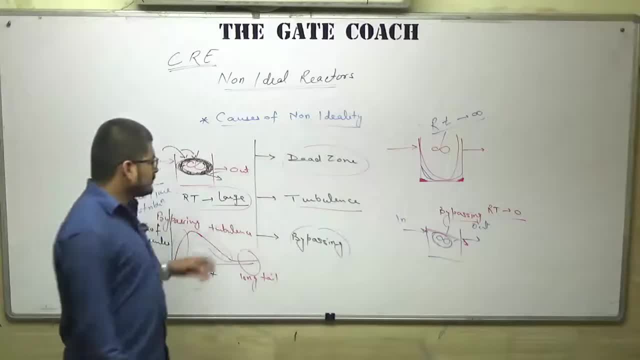 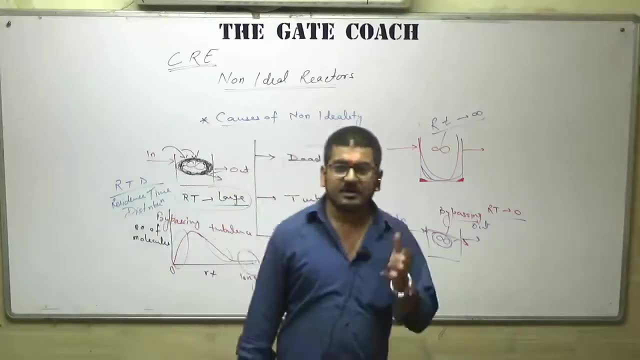 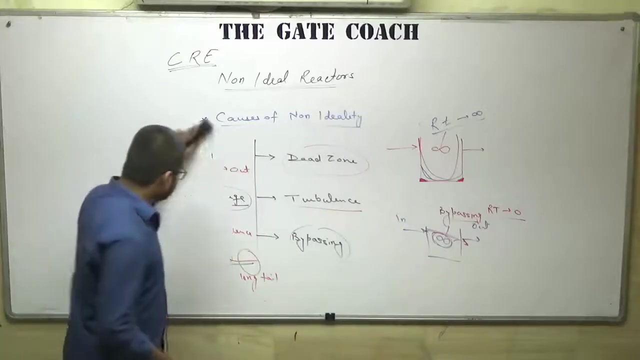 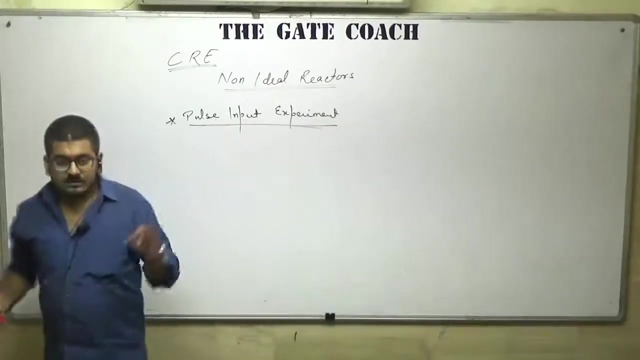 in the class or you can ask me personally, okay, So now I will directly move to the new topic that the input methods of tracer in the reactor. so first- and I will first I will talk about the pulse input experiment. See, guys, as of my experience in this industry from last 5-6 years, this is one of the under 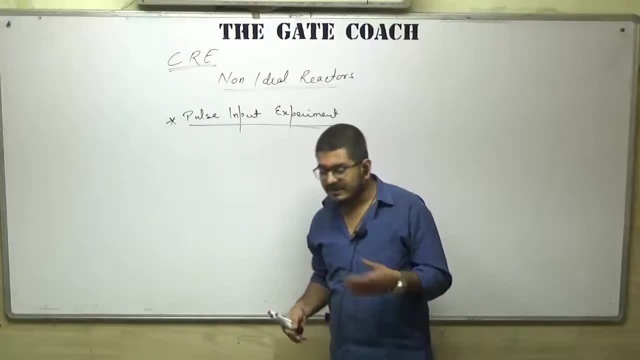 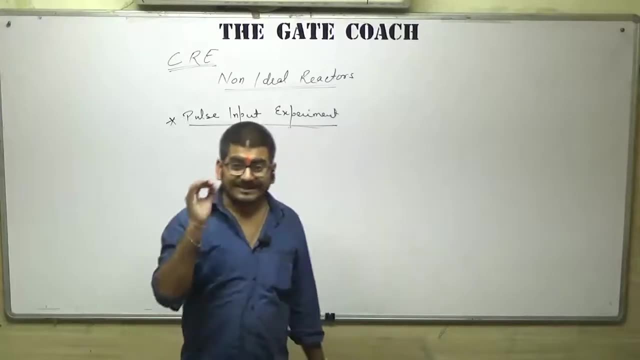 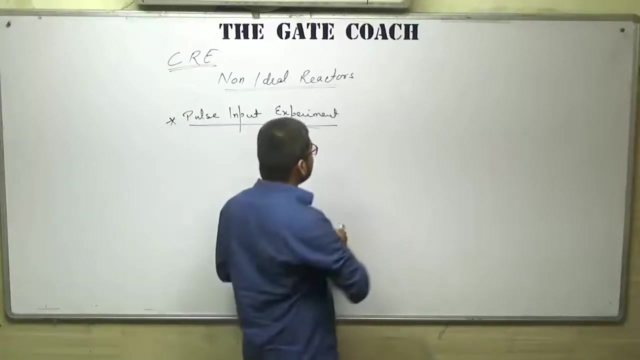 rated topic of CRE because people think it is very difficult- the RTD part. but I tell you that this is the most easy topic of this subject and you can score 100% marks from this topic because every time in gate exam you will get a quote. 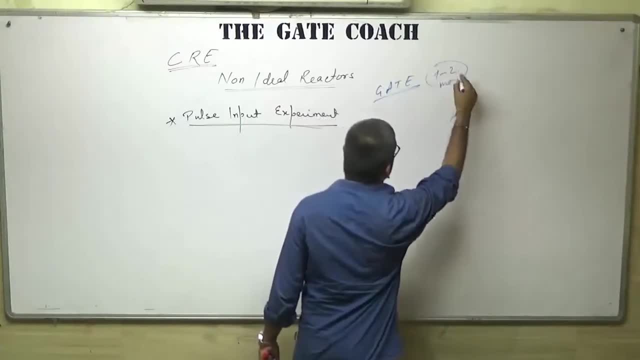 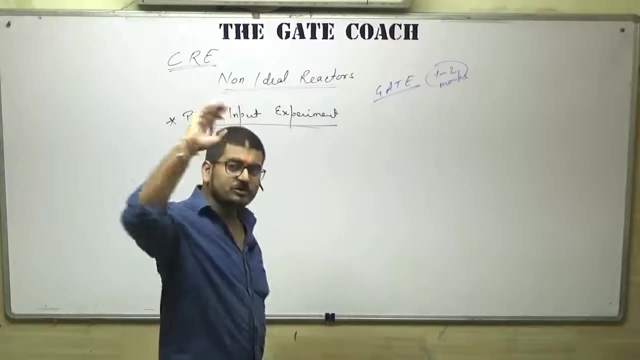 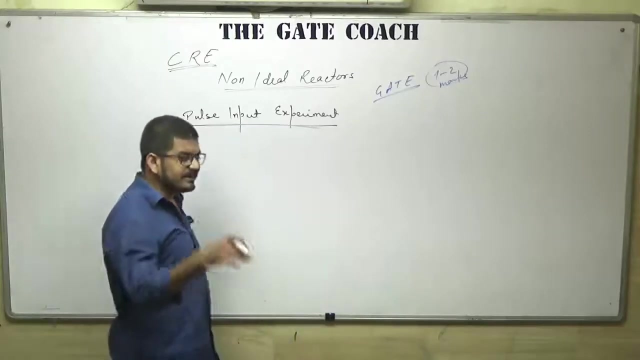 Question from this topic of 102 marks. okay, I don't know why this year there was no question on this topic, but before that, from 2000 to 2017, we were having a 102 question from this topic every time in the exam, and those are very basic and easy question. so if you know, 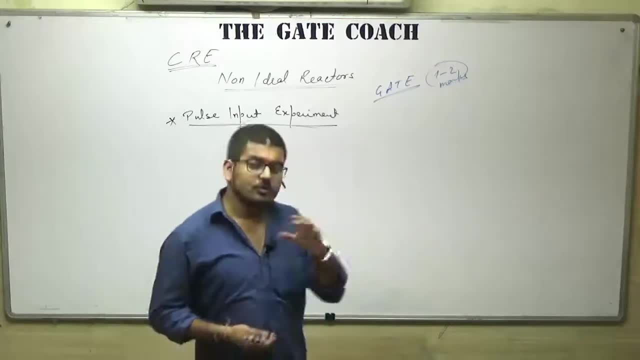 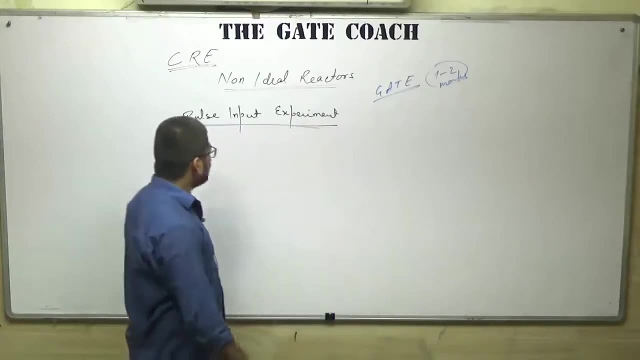 the meaning of each and every term here and you know the basic mathematics of class 10th and 11th, then you can solve any problem of RTD. Okay, how that we will discuss. so pulse input experiment. one point is: what is pulse input? so we know that pulse input is basically the sudden injection, sudden disturbance in the 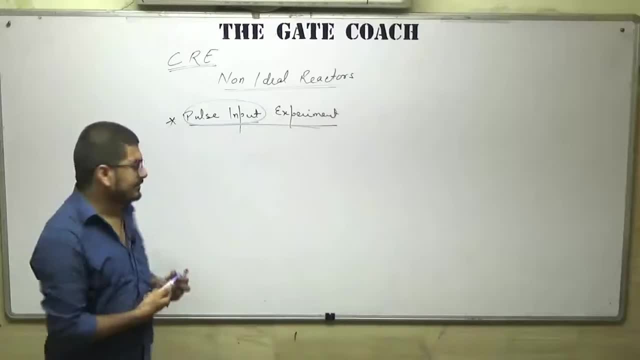 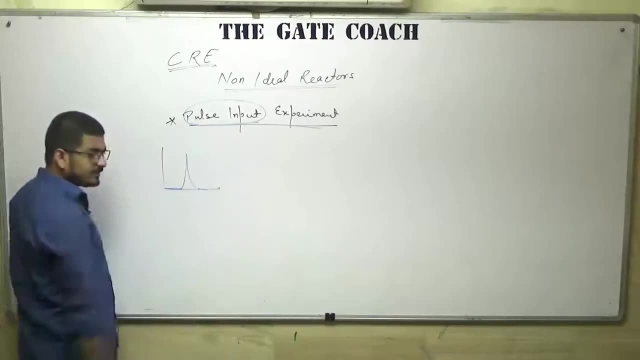 input profile. for a very small fraction of time like this, there is nothing going on and suddenly there is a disturbance, and then again back to 0. so this is, let's say, at t, equal to 0.. This is the tracer inject profile, or input profile we can say to the reactor: sudden pulse. 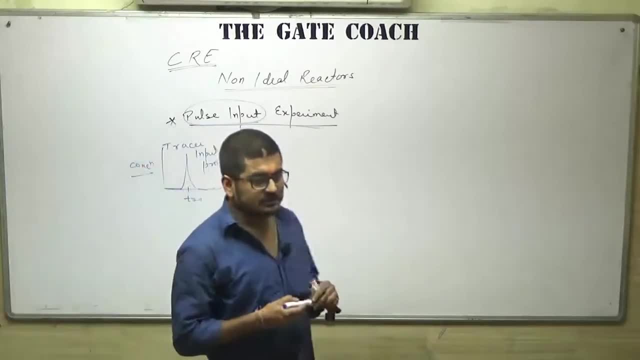 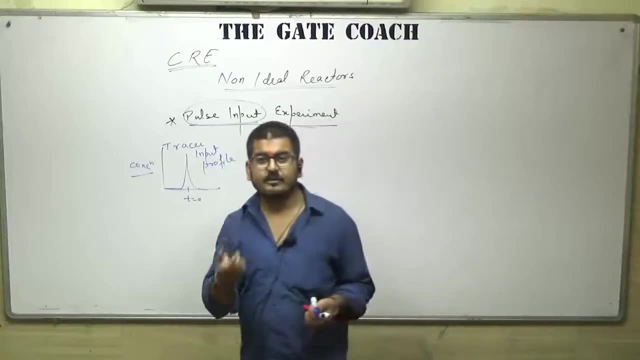 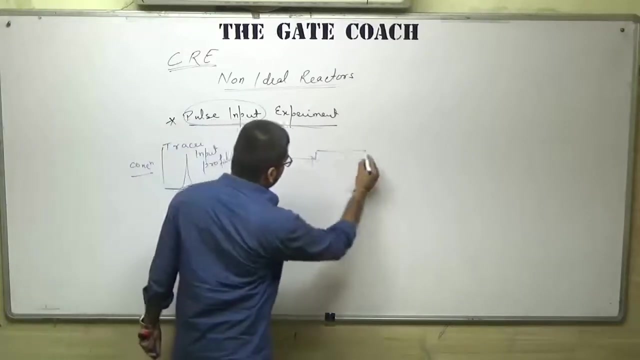 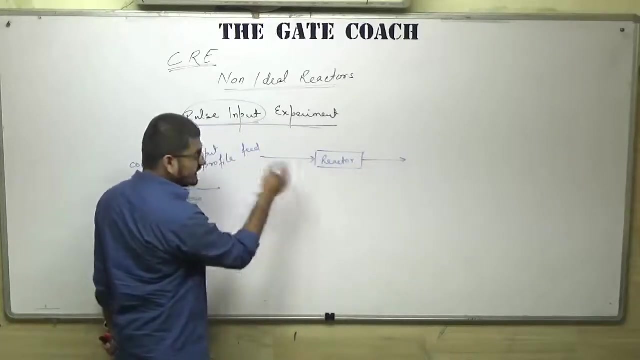 is there. okay, this is pulse input, just like we use to have, we use to inject the serum or any medicine with the help of injection in any human body. okay, so let's say, if I draw a block diagram, Okay, This is the volume of any reactor, so this is the feed going in the reactor with the 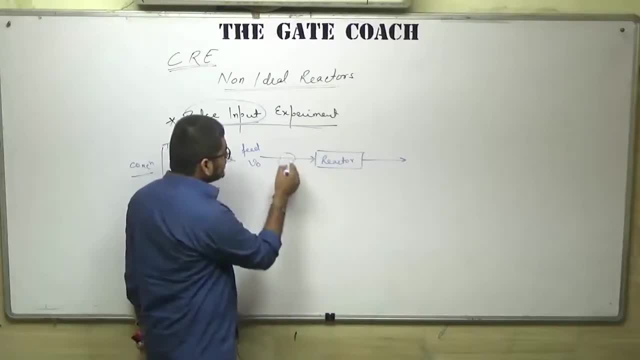 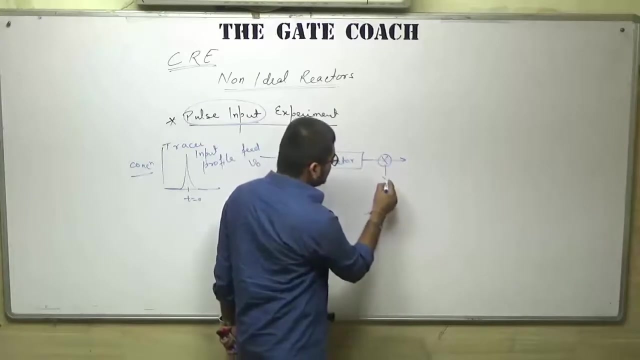 volumetric flow rate V0. and this is the mixing point where I am injecting my tracer at t equal to 0 and at the reactor outlet. this is the detection point. Okay, So this is the reaction point. Okay, So this is the reaction point. 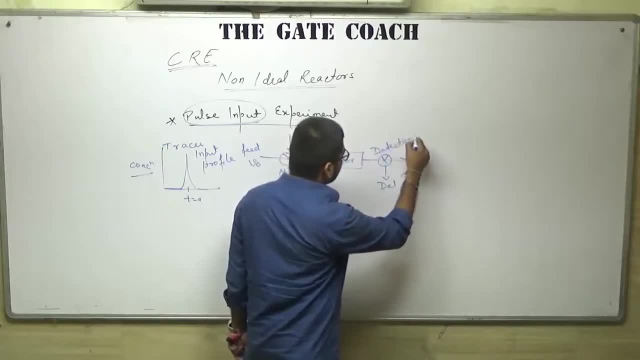 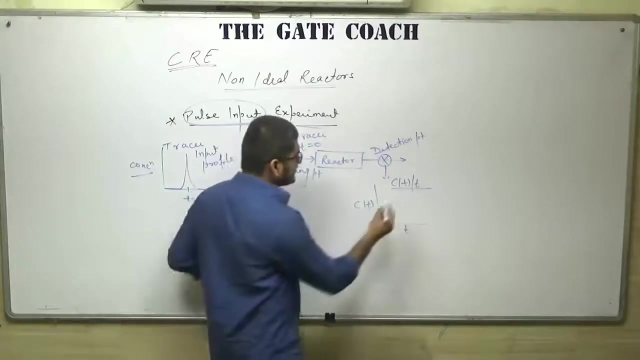 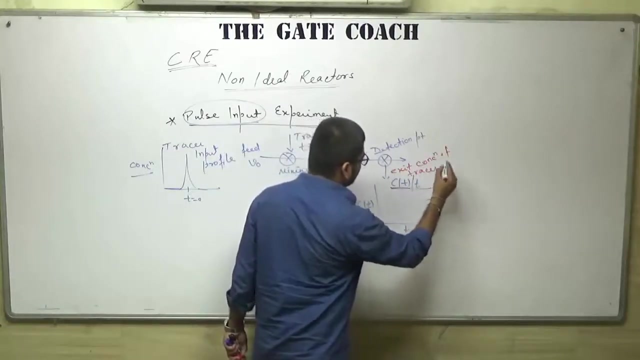 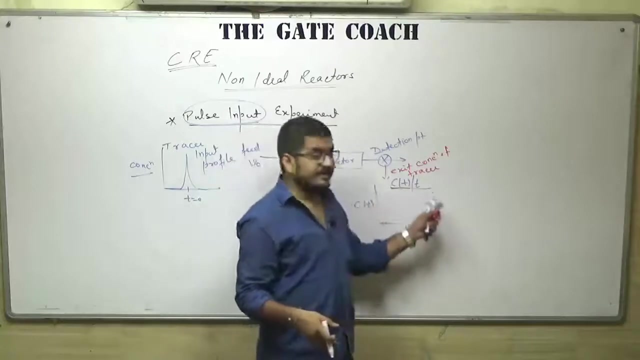 Okay. So this is the concentration of tracer, where I am measuring the concentration of tracer with time. okay, and this is the concentration of tracer. that is basically the exit concentration of tracer Okay With time. So you know that, because of the non-idealities, the exit concentration will be different for 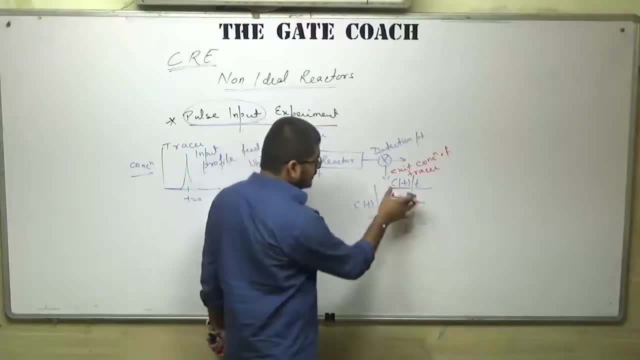 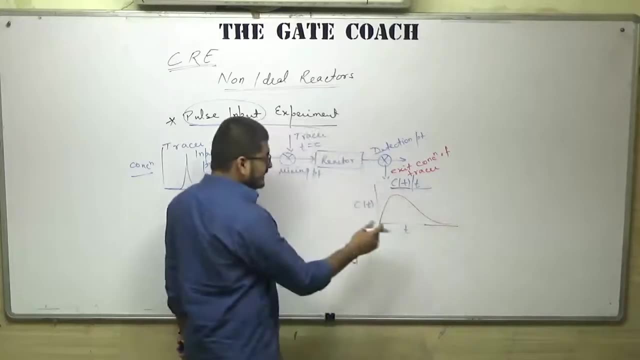 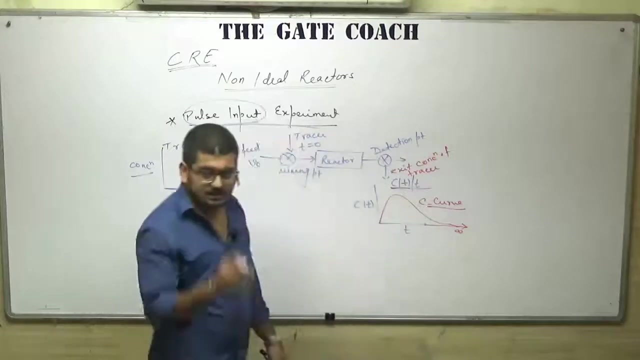 different time period. okay, and when you draw the curve, the curve will come something like this: and the curve drawn between exit concentration of tracer versus residence time for pulse input experiment is known as C curve. Okay, Okay, Okay, Okay, Okay, And at infinite time that curve will touch the X axis means all molecules will leave. 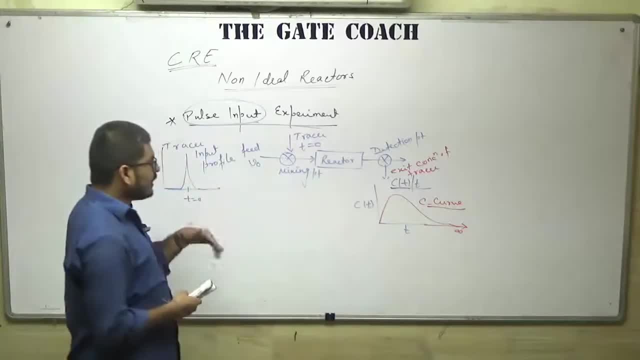 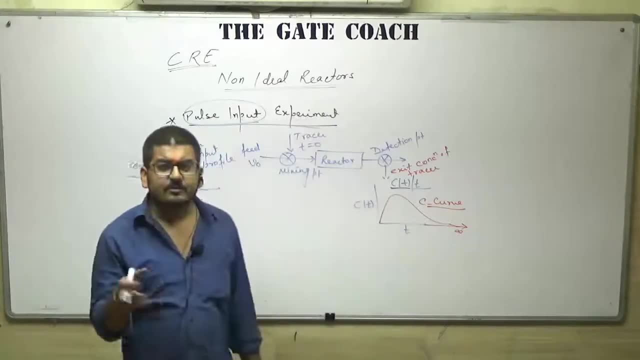 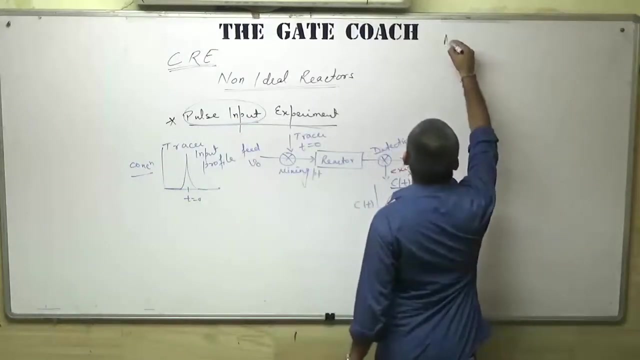 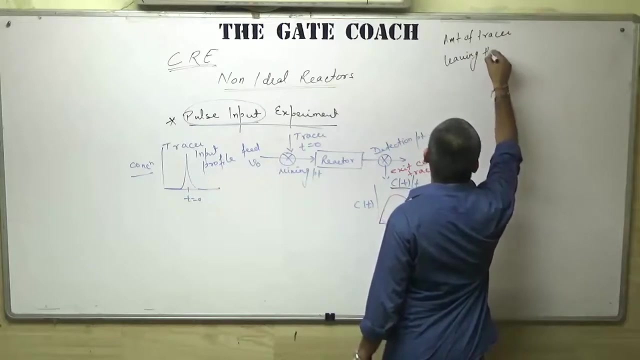 the reactor. Okay, So how to find out that curve and all that we will discuss next is: and all these things we can find out with the help of material balance or mole balance over tracer. Okay, say, we want to calculate the amount of tracer leaving the reactor between time tn, t plus. 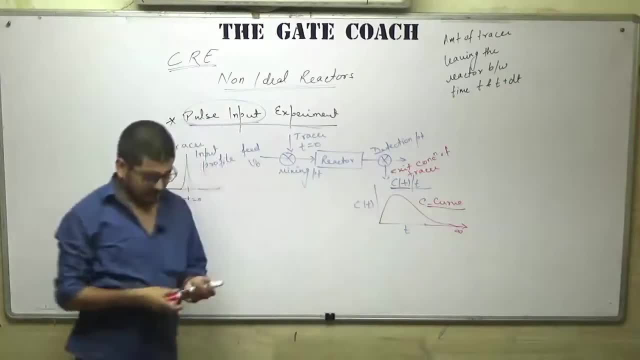 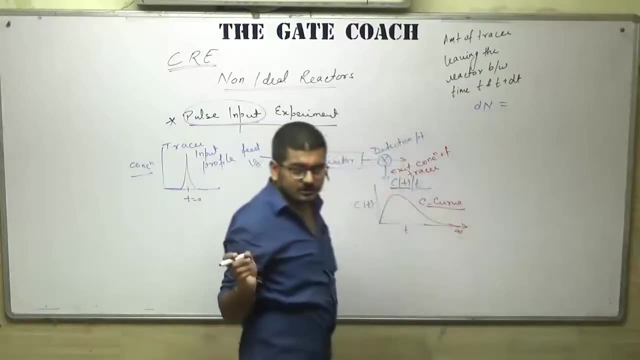 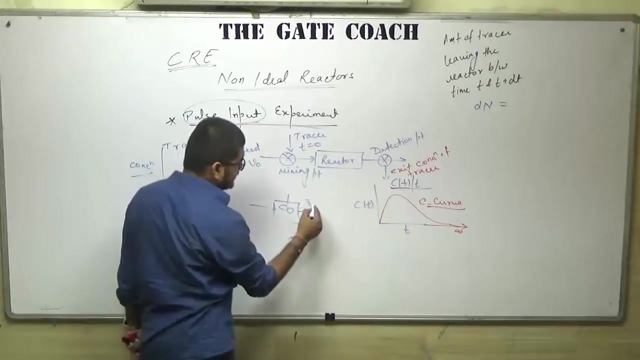 dt and that is, let's say, dn. n represents the number of molecules of tracer, so dn is the amount of tracer leaving the reactor between time t and t plus dt. now see, you know that if there is any tank and the exit flow, exit flow rate is, let's say, 3 kg per minute, then 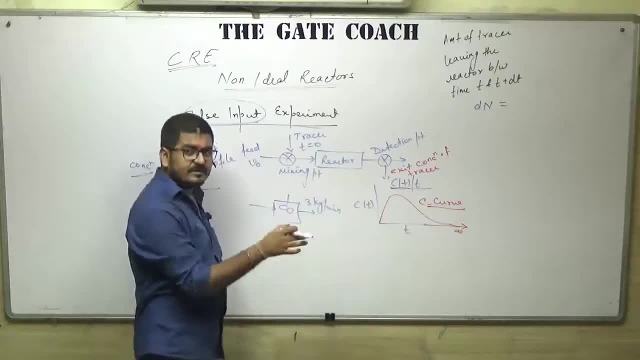 how much amount of this fluid material will leave in 3 minutes. that is 3 into 3, 9 kg, and how much amount of this material will leave between 3 minute and 4 minutes. that is 3 into 9 kg, 3 into 412 minus 3 into 39, that is 3 kg. So in the same way, the amount of tracer leaving. 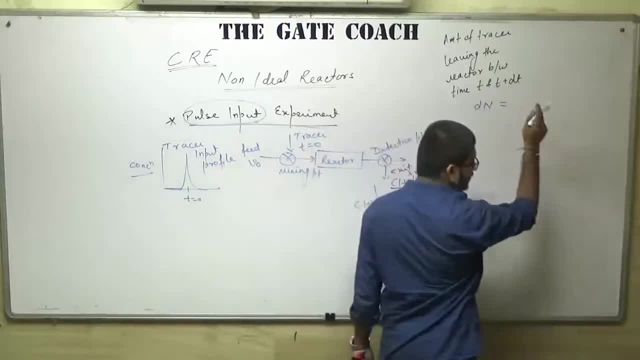 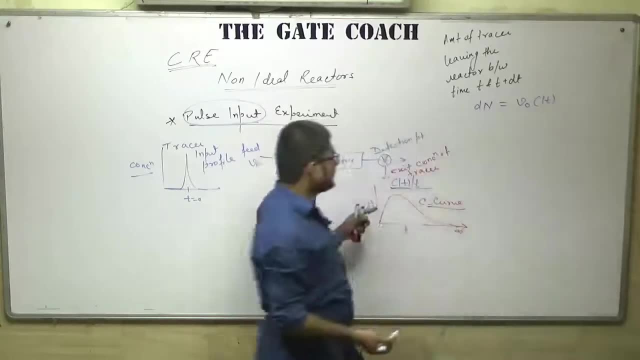 the reactor between time t and t plus dt is the molar flow rate of the tracer at exit. that is the volumetric flow rate multiplied by exit concentration of tracer. So it is molar flow rate of tracer at exit and this reactor is operating at a steady state. so 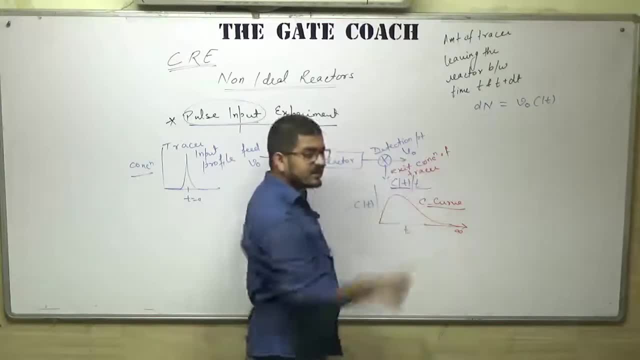 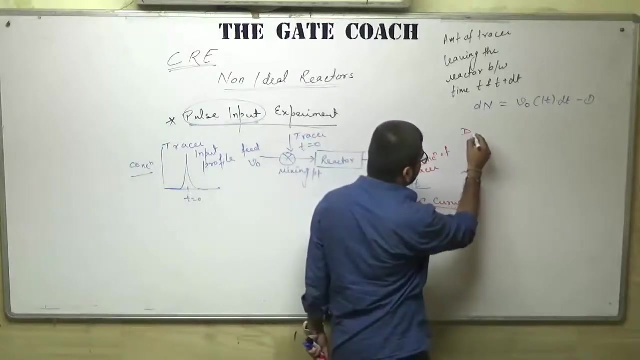 that is why the outlet volumetric flow rate will be V0 as well, multiplied by the time interval, let's say equation 1.. So this is the amount of tracer leaving the reactor between time t and t plus dt. and let's say, if we divide this and by N0, that will be like dN over N0. 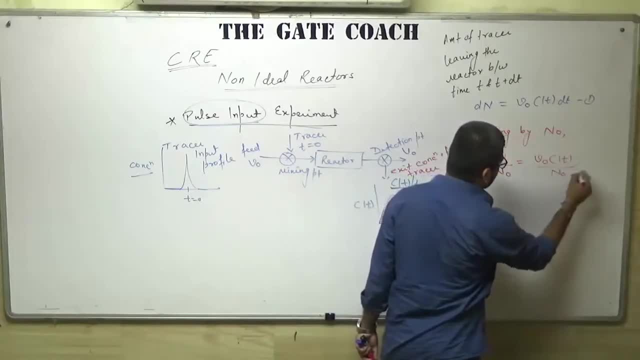 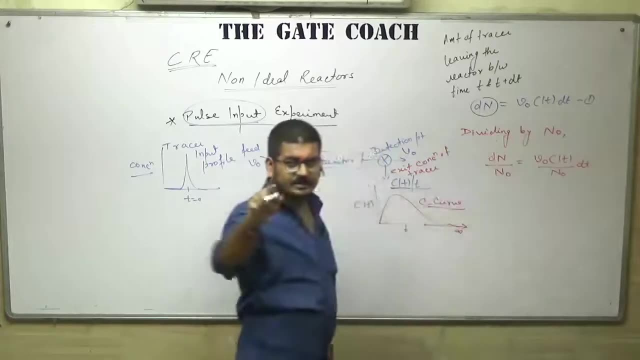 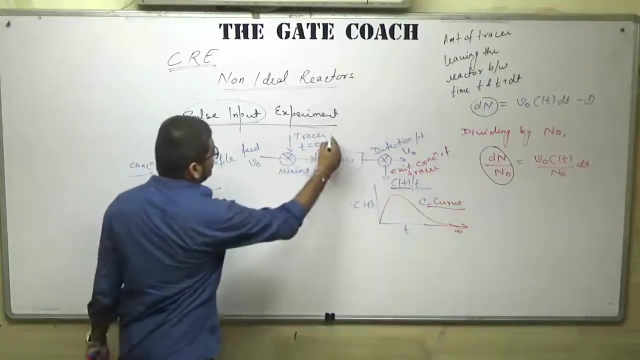 is equal to dN over N0, is equal to dN over N0, is equal to oiz. find dNs, my and dN is the amount of tracer leaving the reactor between time t and t plus dt. so dN over N0 and N0, which is the total amount of tracer be injected in reactor. 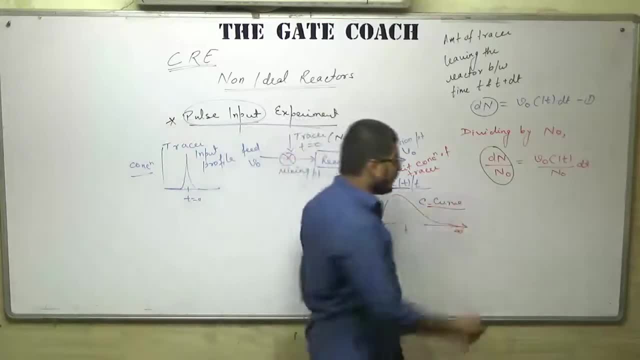 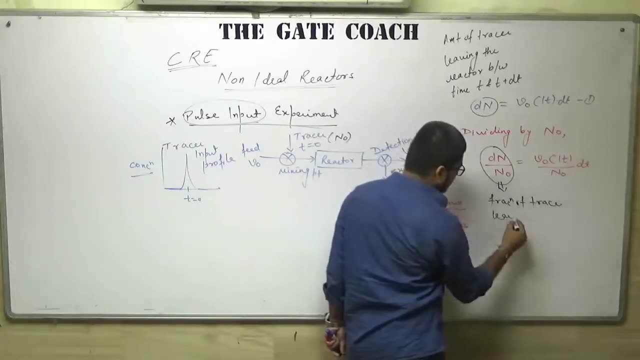 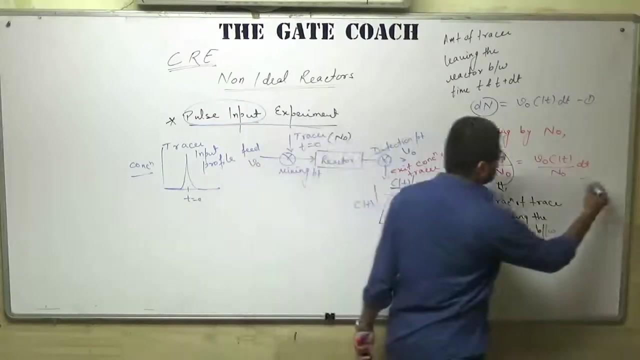 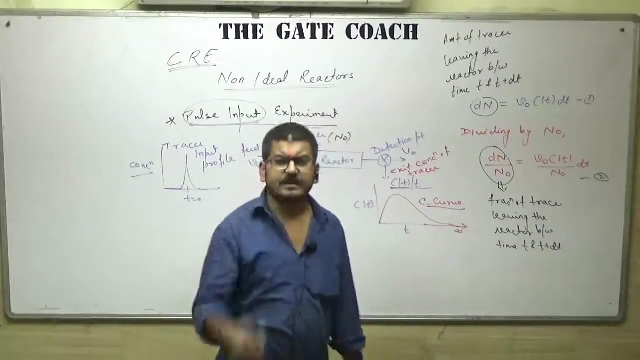 So amount leaving the reactor divided by total amount, it will what fraction of tracer leaving the reactor Ld Vl between time t and t plus dt, let's say equation 2. and I believe that in statistical mathematics you have studied about the probability distribution, binomial distribution, Poisson distribution. 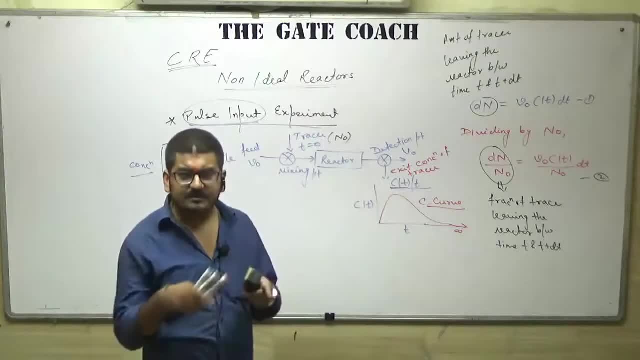 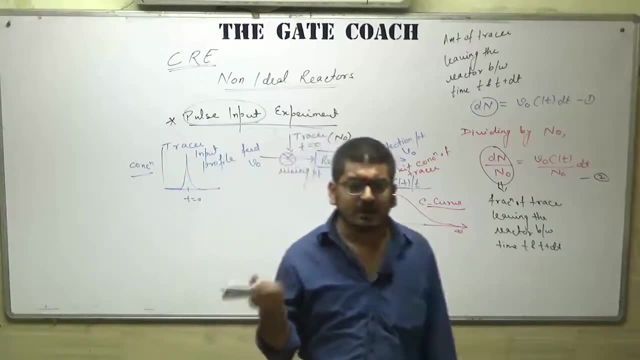 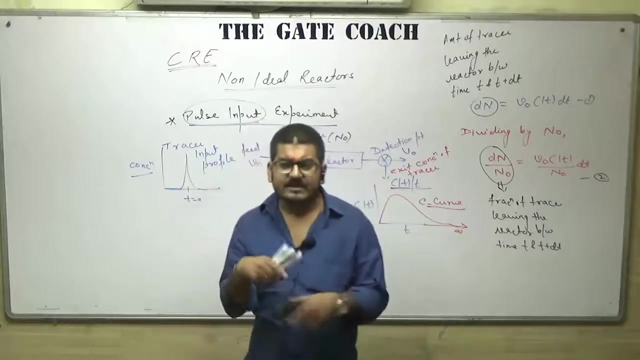 and normal distribution, etc. so in all of the curves, when we analyze the distribution curve, there was one thing common: that we want to find out the mean value, median and mode, standard deviation and variance of the curves, and all these things, all these parameters. 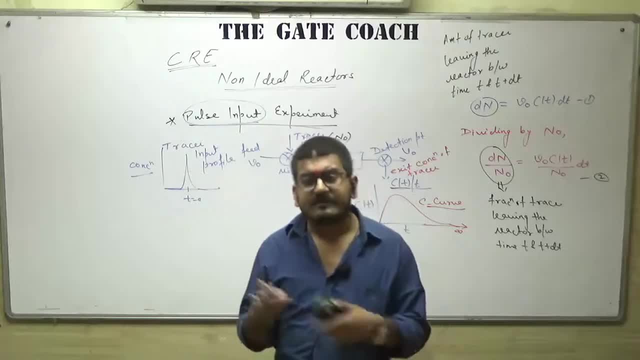 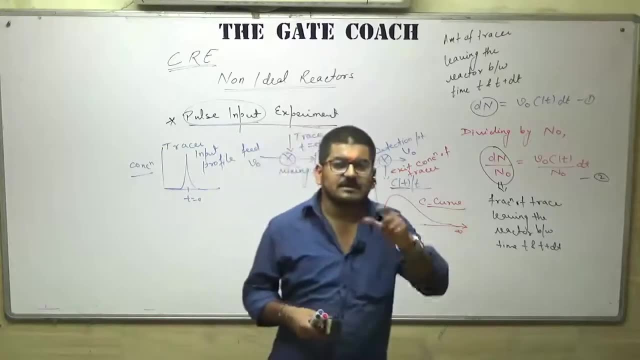 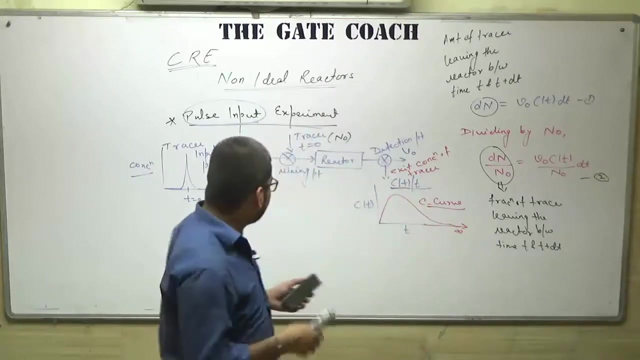 we calculated or we calculate with the help of some distribution function there. so, in the same way, this residence time distribution is basically the application of the distribution, of probability distribution. all these things are based on probability distribution, but we will not talk about that because this is not the math class, this is the CRE class. 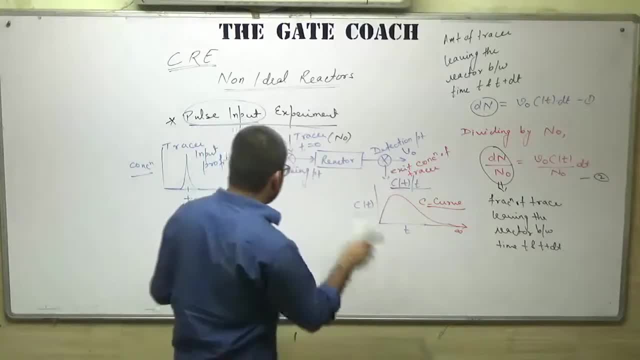 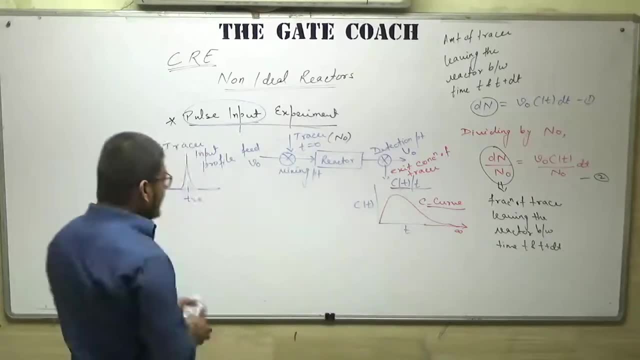 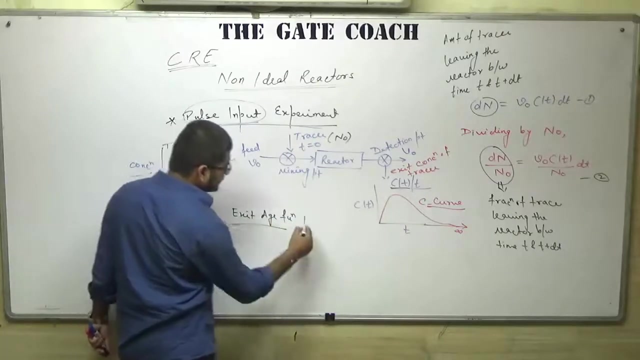 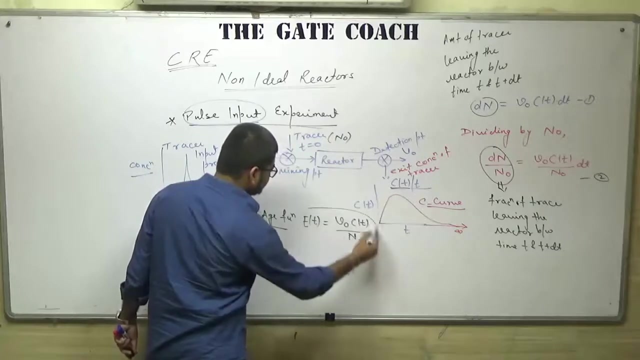 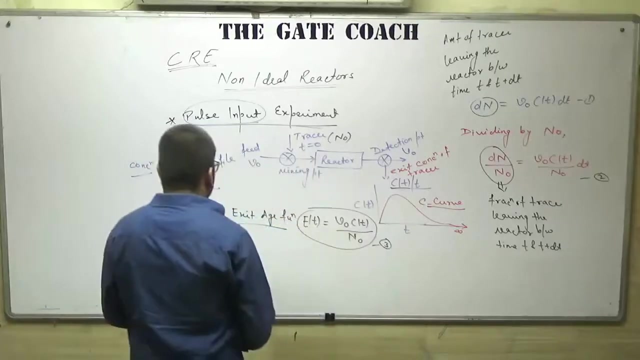 so we will discuss that thing, how to use that. so here as well, for this C curl, we will find out. we will define a distribution function known as exit h function, Which is like P0 into multiply by Ct divided by N0, let's see equation 3, okay, and what? 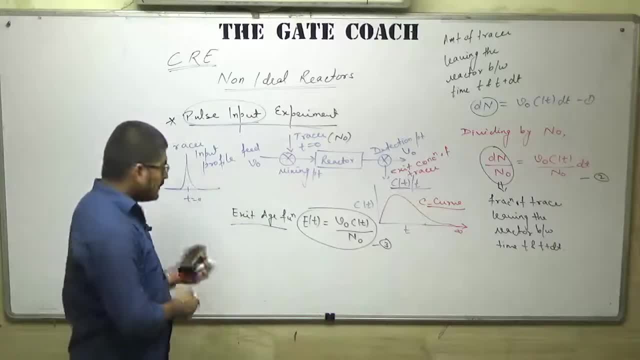 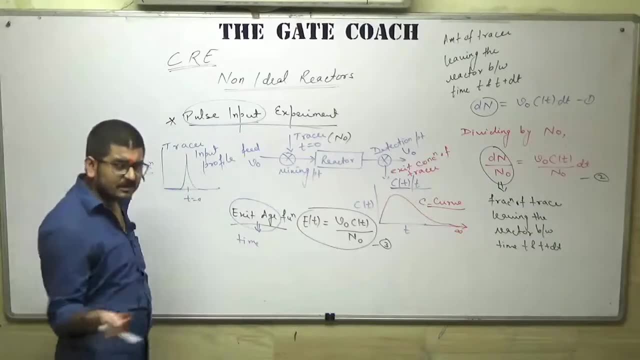 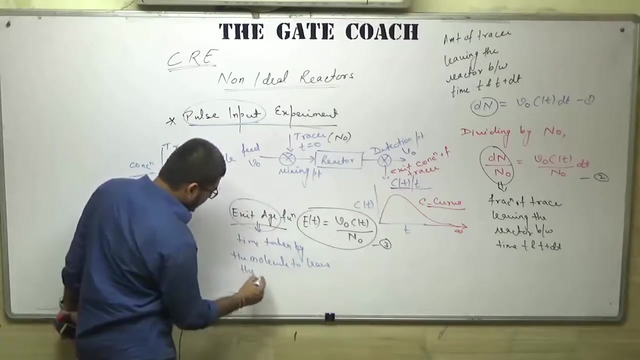 is exit h. so exit h is. it is just analogous to the residence time, but definition wise, we can say it is the time taken by the molecule Right To leave the reactor, time taken by the molecule to leave the reactor. so now see, it is just. 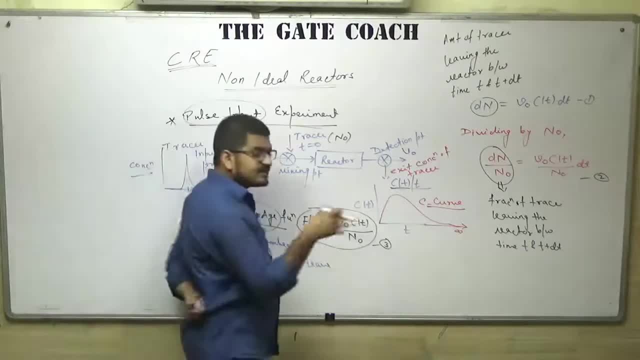 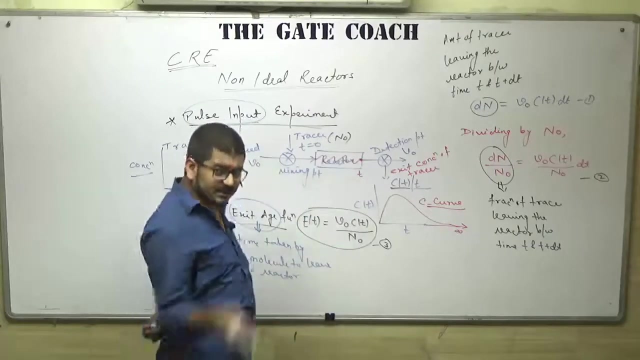 like the residence time. here residence time can be defined as the time spent by the molecule within the reactor. so when the molecule entered in the reactor, that is t equal to 0, and when it leaves the reactor, at time t, that duration we call residence time. but in the same way 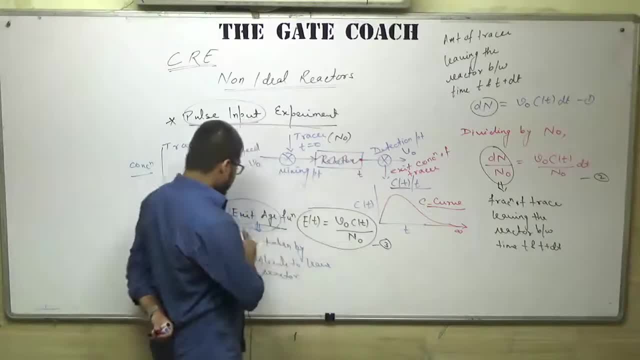 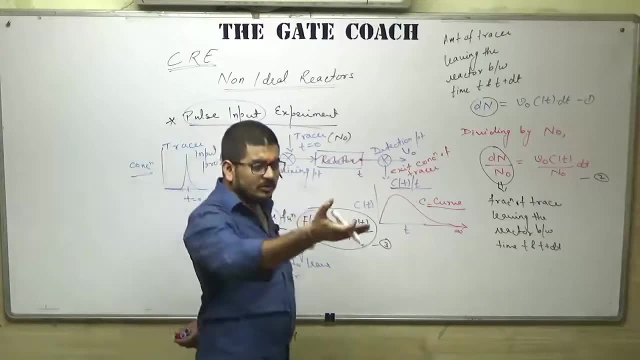 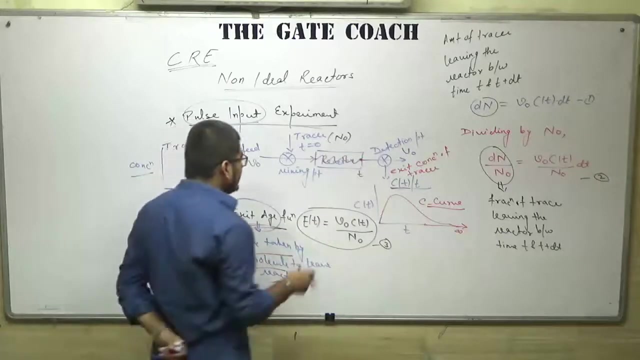 here in exit h function. exit h Right, Which is the time taken by the molecule to leave the reactor, means we are waiting at the outlet to leave the. we are waiting at the outlet of reactor for the molecule to leave. okay, so what we are doing, as you can see in this experiment, we are injecting the. 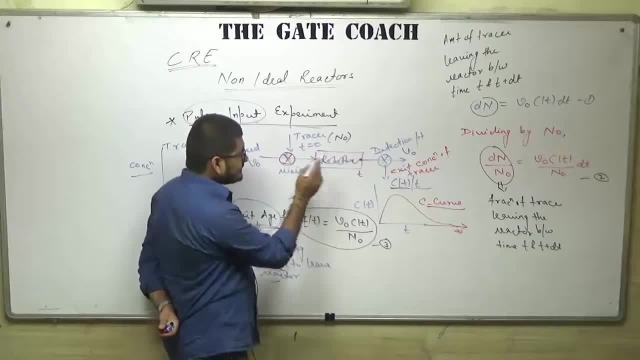 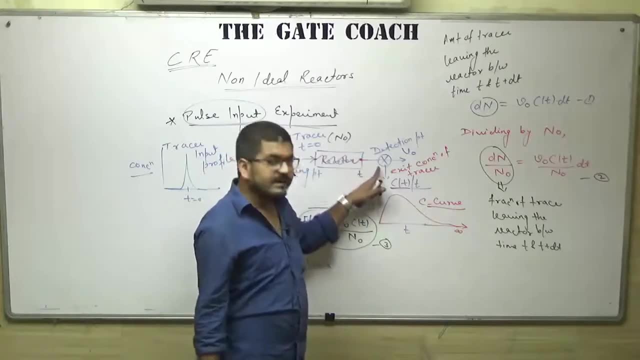 tracer at time t equal to 0 and it enters in this. okay, now we are waiting at outlet for the molecules to leave. And when the molecule will leave, We will calculate the time Right. We will measure their concentration with the help of titration chromatography or n number. 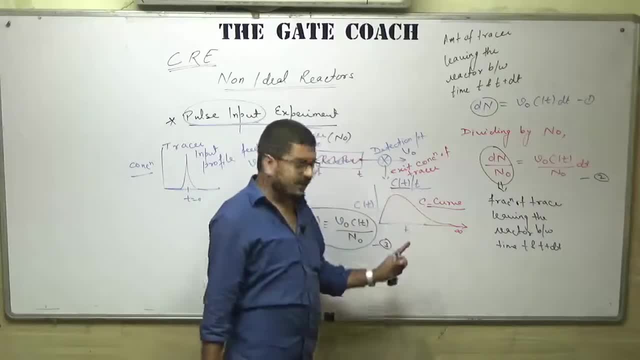 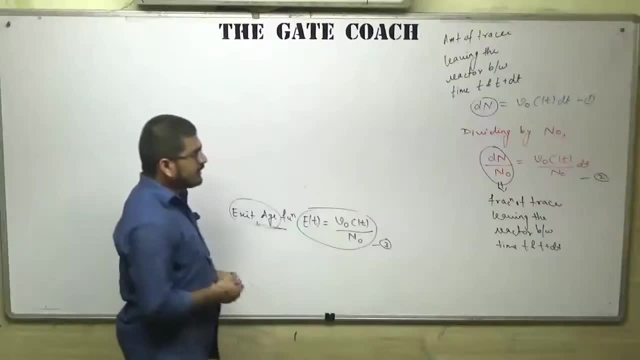 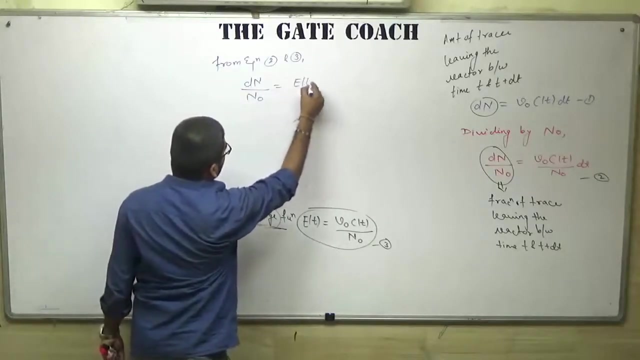 of phase are there and we will draw the curve. okay, and this is what we call exit h- time taken by the molecule to leave the reactor. okay, So from equation 2 and 3 it is clear that dn over n0 is equal to et into dt. okay, and 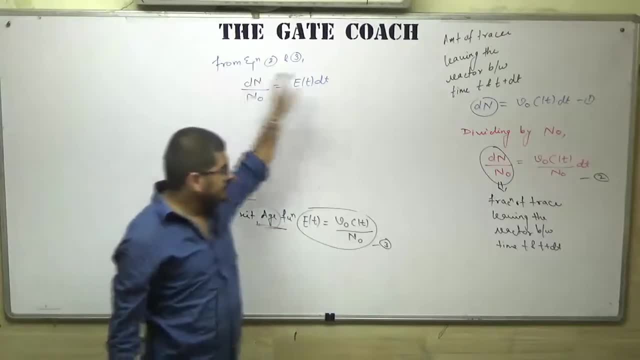 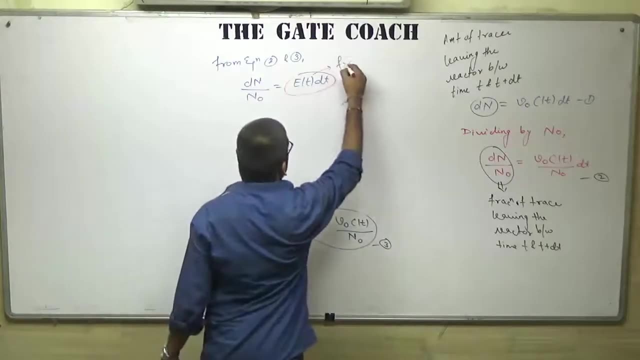 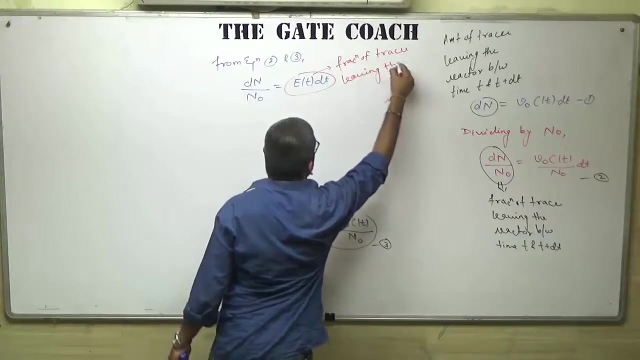 what is dn over n0?? Okay, The fraction of tracer leaving the reactor between time t and t plus dt. so in the same way, this et dt will also define as the fraction of tracer leaving the reactor between time t and t plus dt. okay, 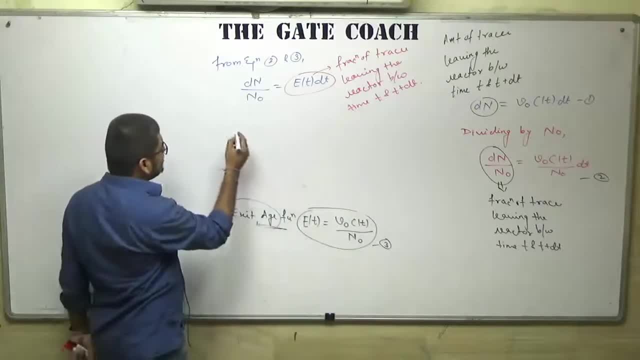 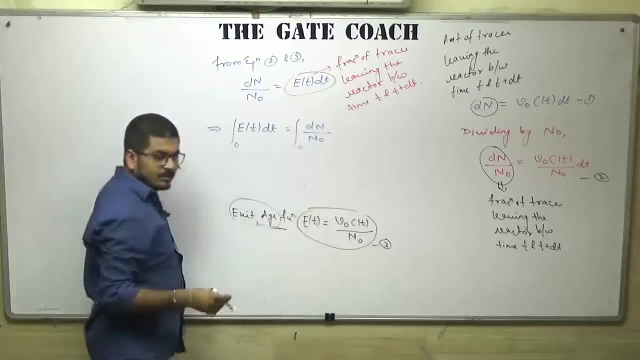 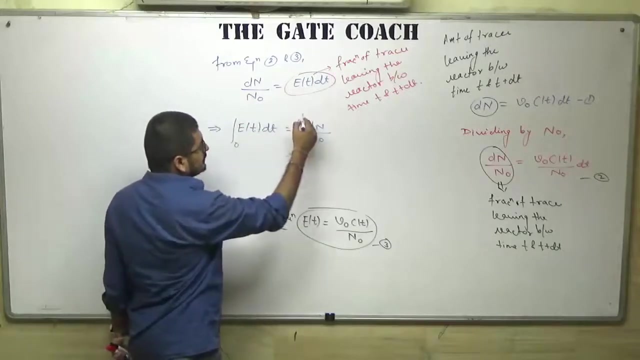 Okay, Okay. So if you integrate this point, so at time t equal to 0, the molecules leaving the reactor will be 0, because at 0 we are injecting some molecules, so they will not leave, and the time required by the molecules, the time at which all molecules will leave, will be infinite. 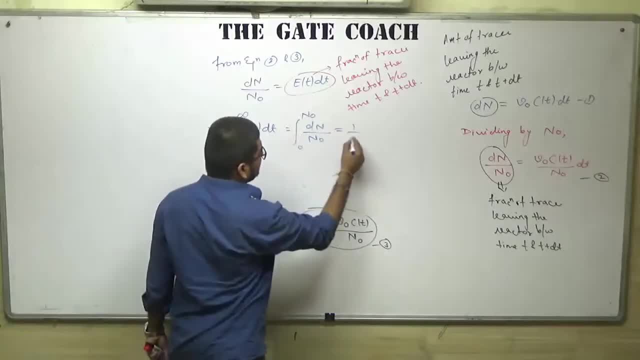 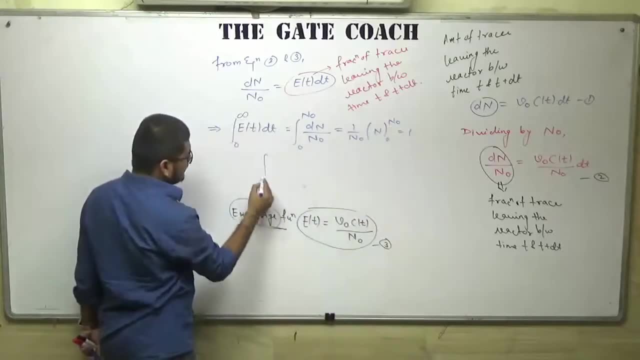 because of the dead zone, and when you solve this it will be like: Okay, So you can write it as 0 to infinite. et dt is equal to 1,. okay, and let's say this is equation 4, et dt was fraction of tracer leaving the reactor between time t and t plus dt, and. 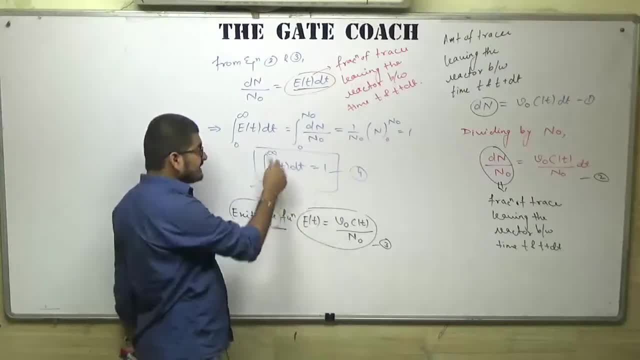 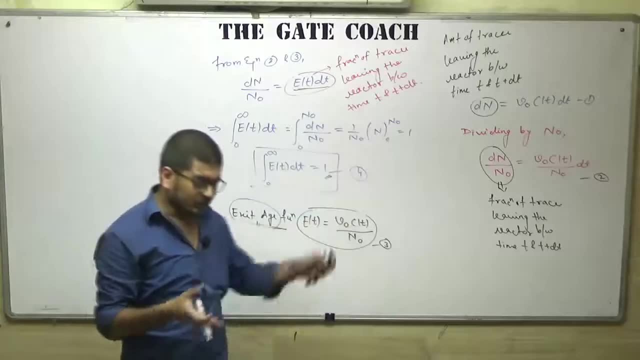 when we integrate this from 0 to infinite means in total time interval, the fraction of tracer will leave the reactor. So the fraction of tracer leaving the reactor will be 1, and it should be 1, obviously. In total time interval, all molecules will leave the reactor, so the fraction will be 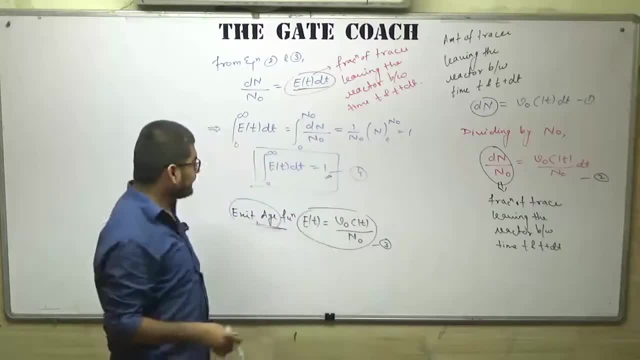 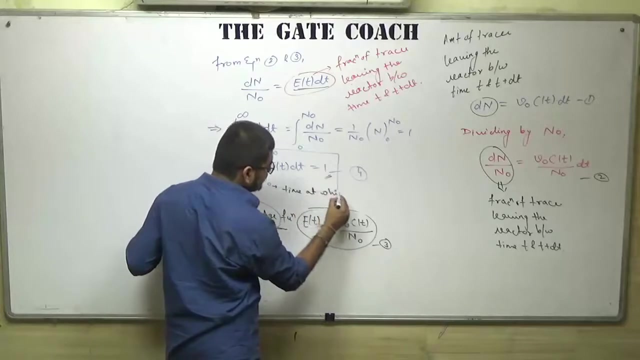 1. So this is correct, okay, and here the 0 is the time at which molecules. here the meaning of this: 0, the initial limit is the time at which molecules have started. Okay, Okay, Okay, Okay, Okay. 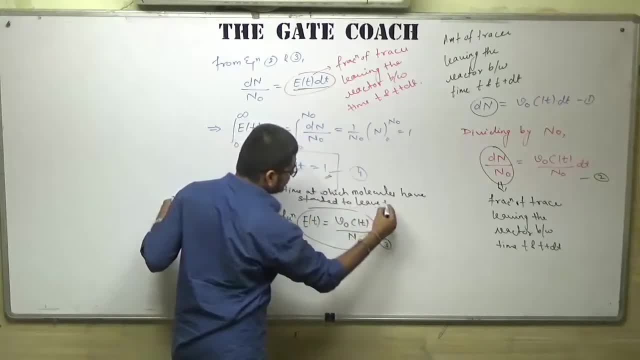 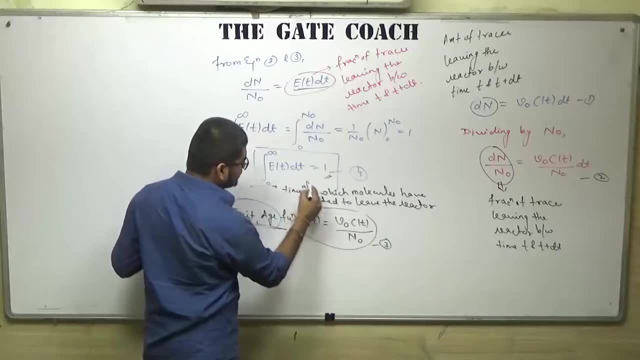 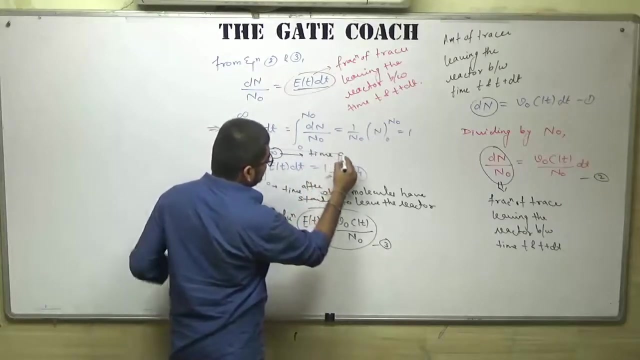 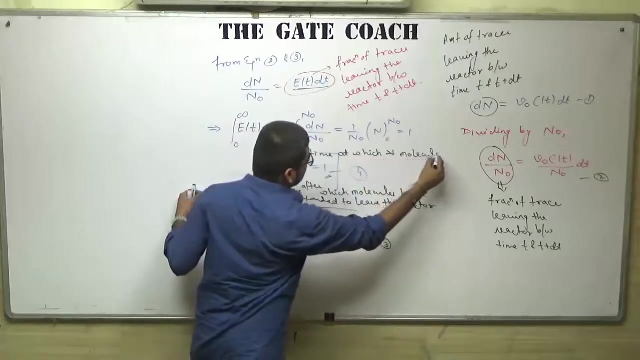 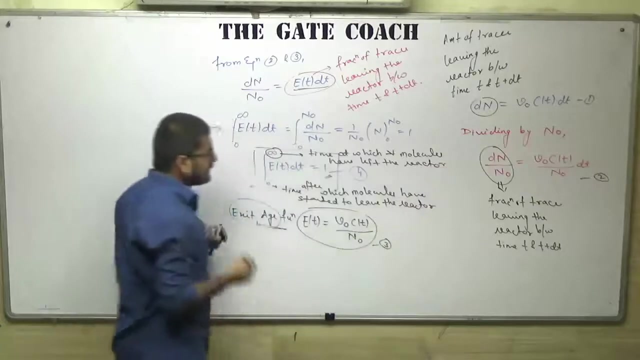 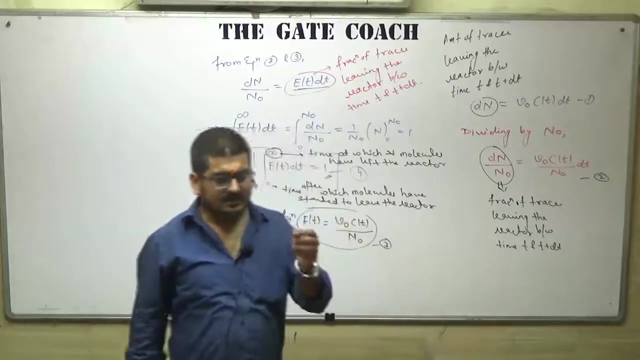 Okay, Okay, To leave the reactor. Okay, Okay, Okay, Okay. Actually, time at which means time after which- Okay, and the infinite it means the time at which all molecules have left the reactor. Okay, That is not the 0 and infinite, it can be also 3 and 25,. there is a reactor at t equal. 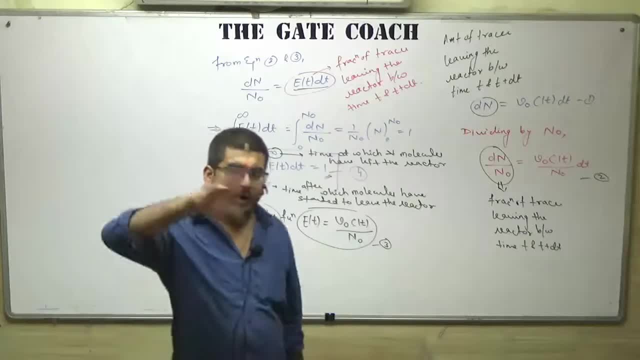 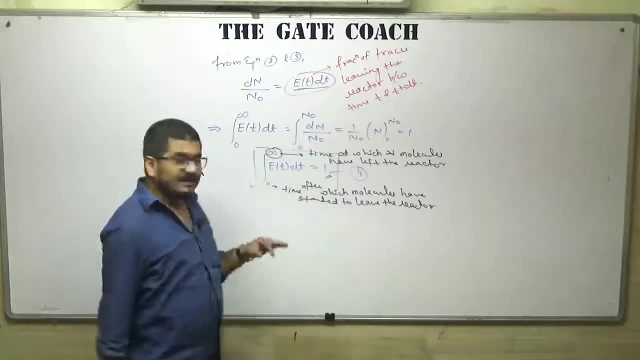 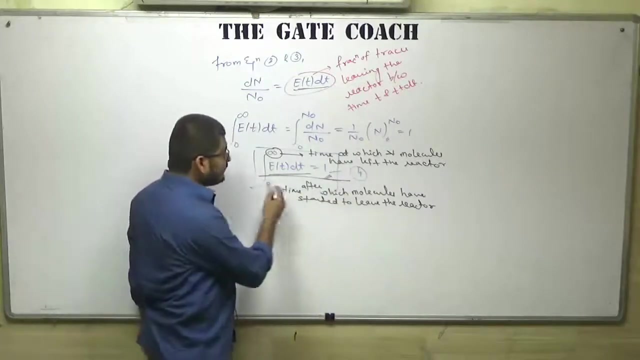 to 3 minutes, molecules are started to leave and all molecules will leave till t, equal to 25 minutes. so the limits will be like that. I think it is clear to all of you. then now see this equation 4,. this represents one more meaning, as all of us know: the application. 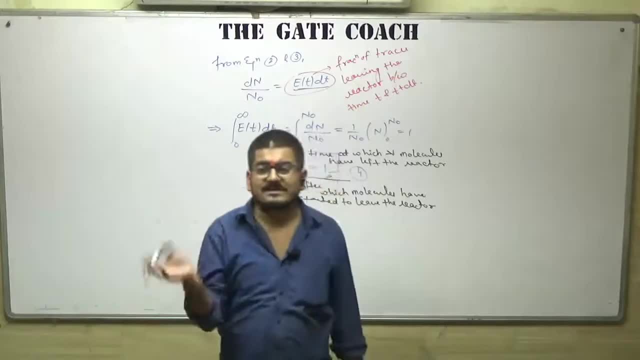 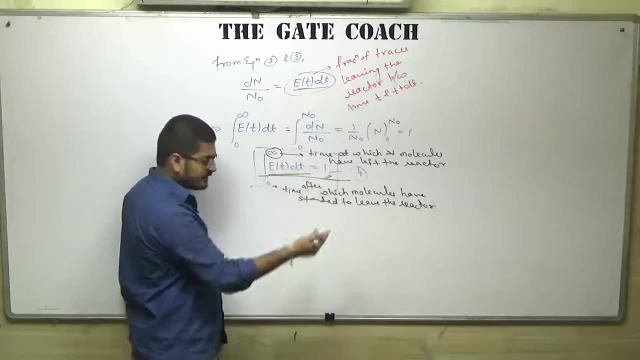 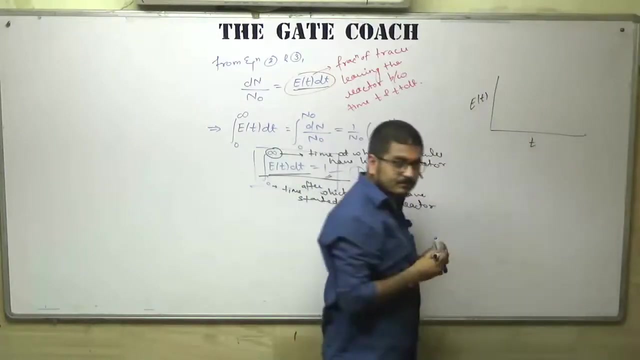 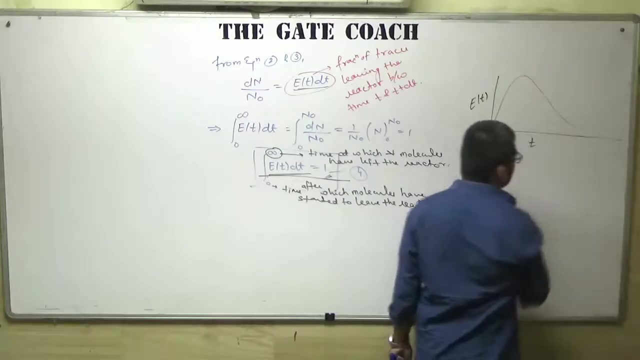 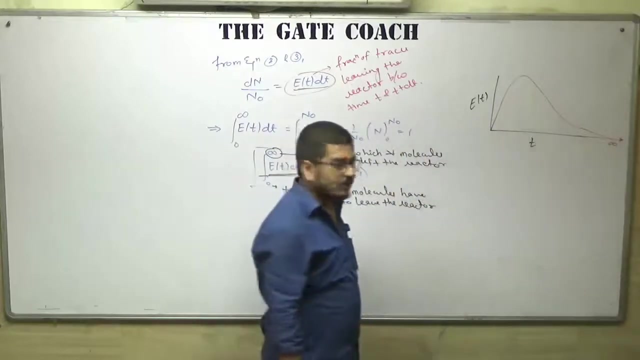 of integration is. it also represents the area of some function means in this curve. it represents the area of this e versus time curve. so if we draw a curve between e versus time, so it will be like this And this curve will leave at t equal to infinite, will touch the x axis in the curve drawn. 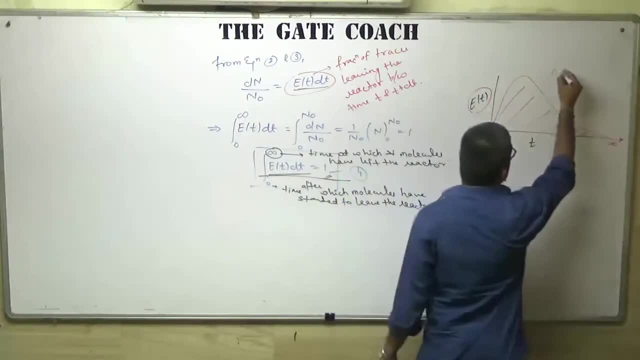 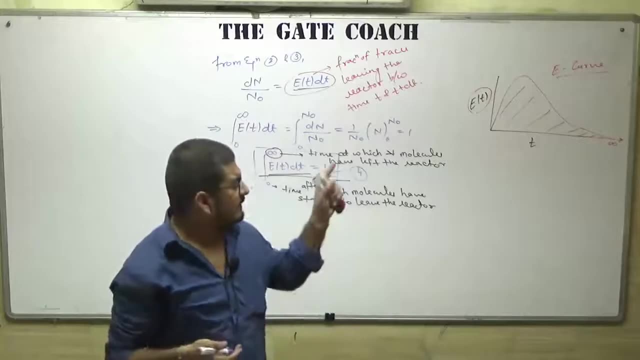 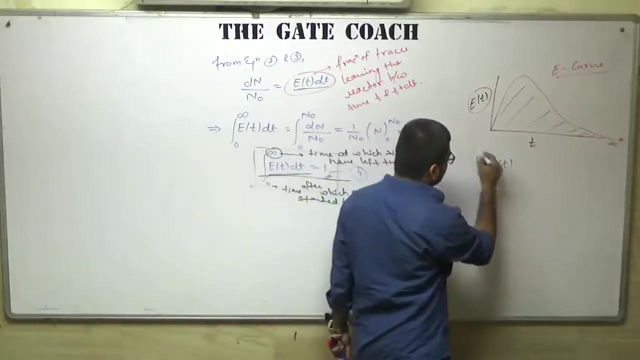 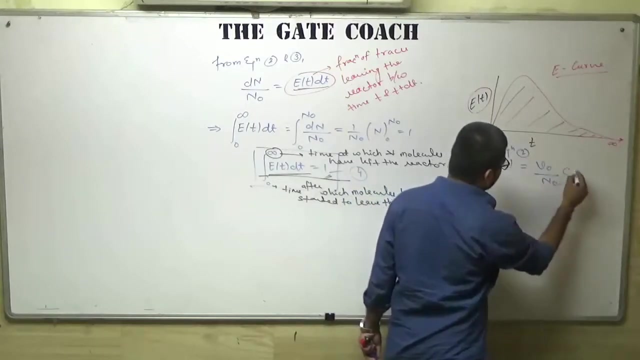 between e exudate function versus time is known as e curve. now I think you will think that why the shape of this curve is like this? so if I say that, remember equation 2, this equation from equation 2, E t was like V 0 over N 0 multiplied by C, t and the C curve. 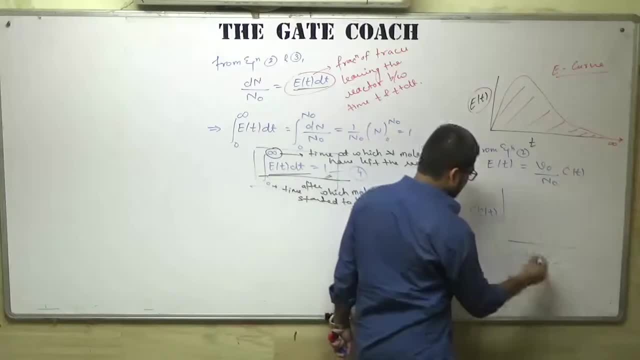 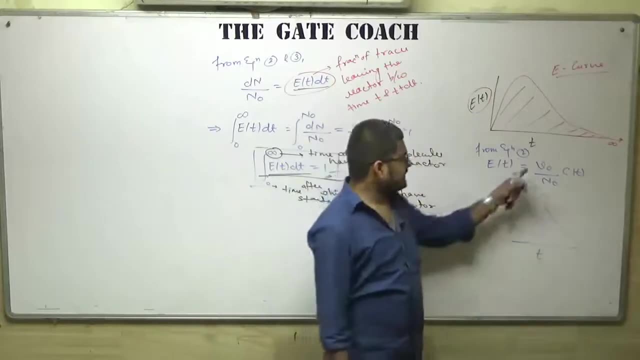 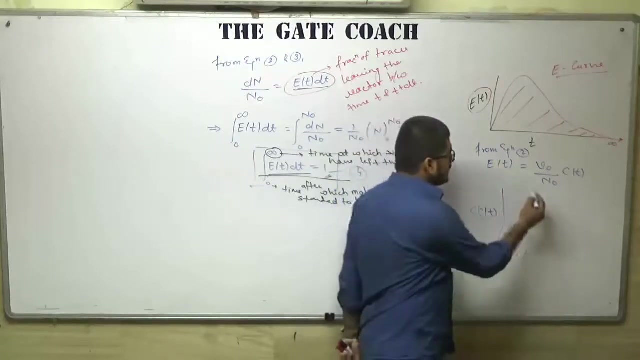 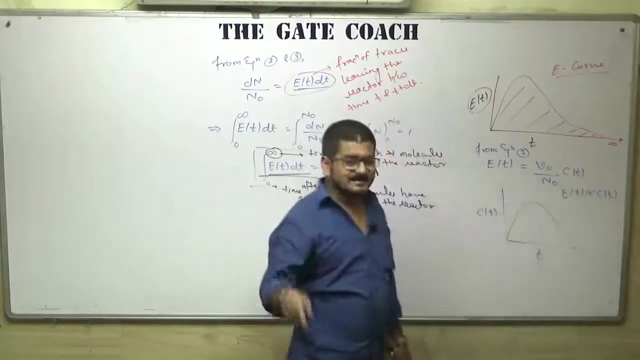 was like this. so you can see, V 0 is constant because the steady state reactor is there. N 0 is the total amount of tracer molecules, which is already constant. so we can see this. so E t is like a half energy Cuban curve. how will we have E t? 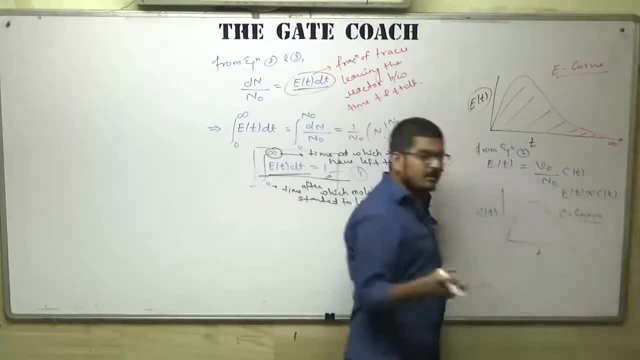 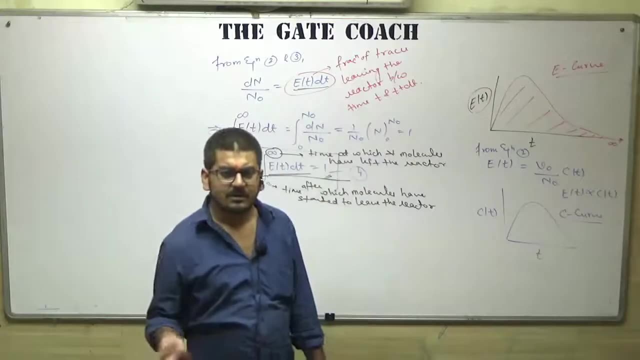 I will say that. let me understand a bit, isn't it? You will get the ratio of 1.ệC to Sn square we need to constru, or you will also get sen square, anc x, 0 and anc. 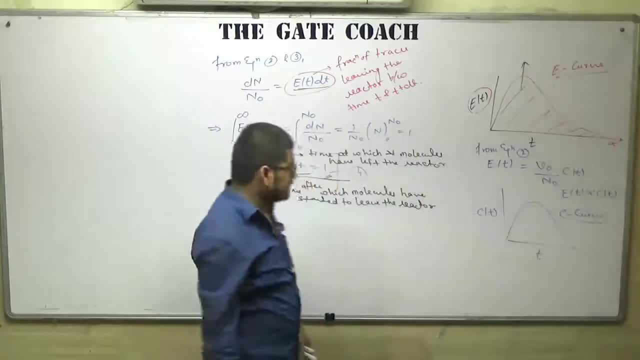 x 2 are similar, golden and all also the same, and then say: right now, this is the original equation. we will see that h is not equal to ne, e equal to ne dzi, nmd max ne znp. 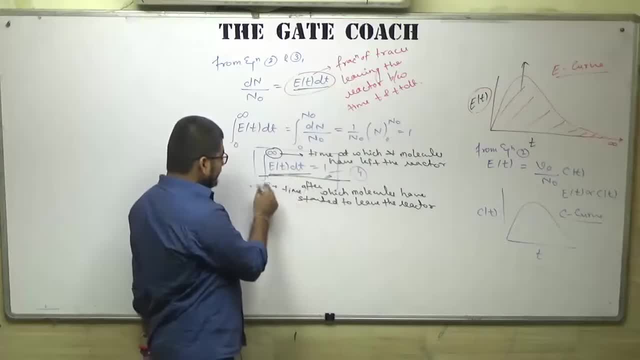 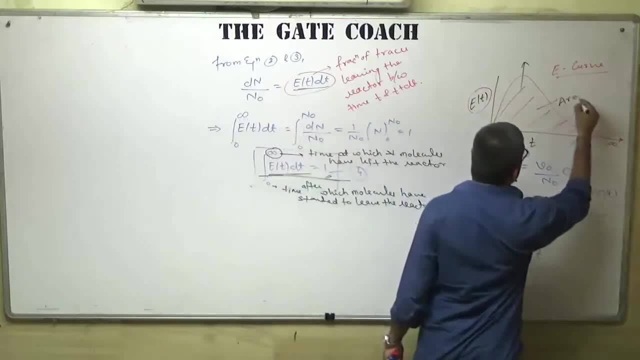 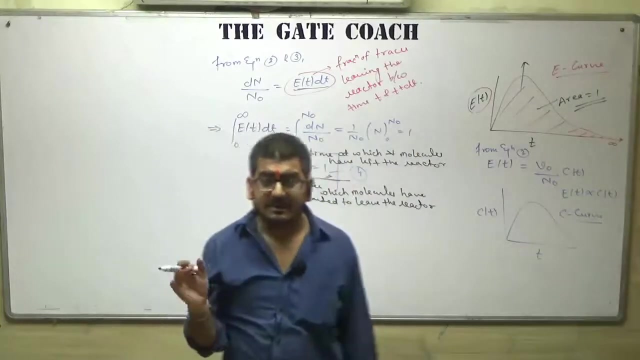 can see from this curve, this equation 4, that from limits 0 to infinite, means in total time interval, the area of this curve will always be 1. okay, so remember this guys, this is a very key point in this study- that area of E curve will always be 1 for the total time. 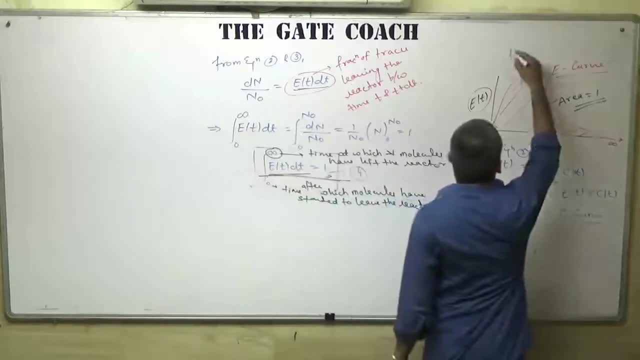 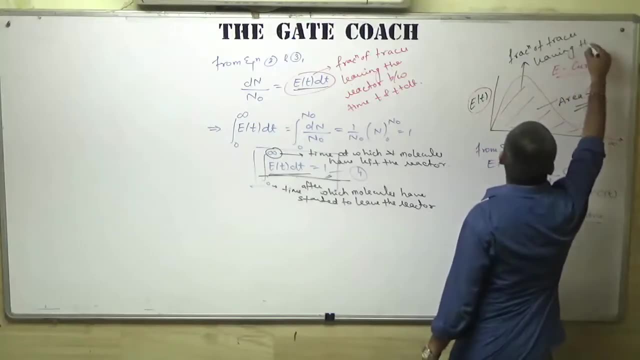 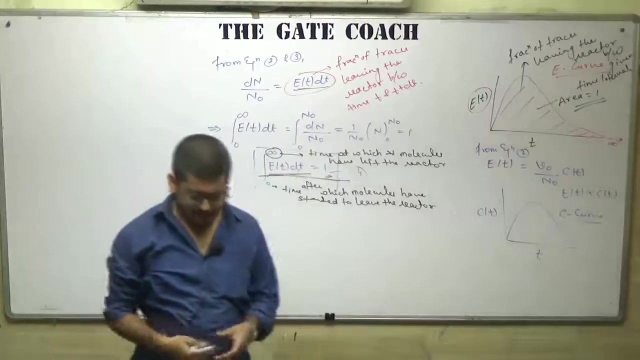 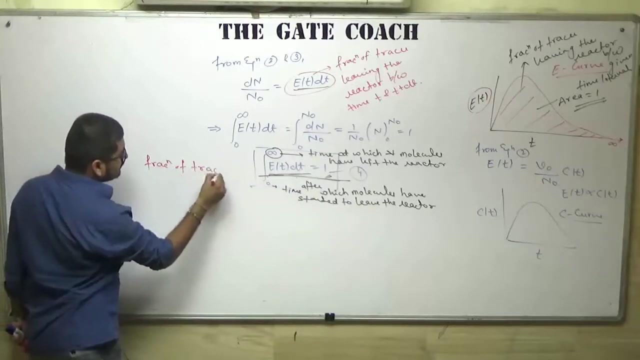 interval. okay. and the area of E curve represents the fraction of molecules, fraction of tracer leaving the reactor between given time interval, okay. so if someone ask you to calculate the fraction of tracer leaving the reactor, okay. so if someone ask you to calculate the fraction of tracer from the distribution of burned, hissing residents for 10 years, what should be calculated in? 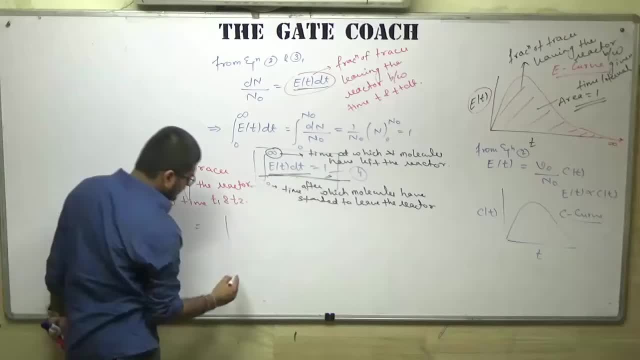 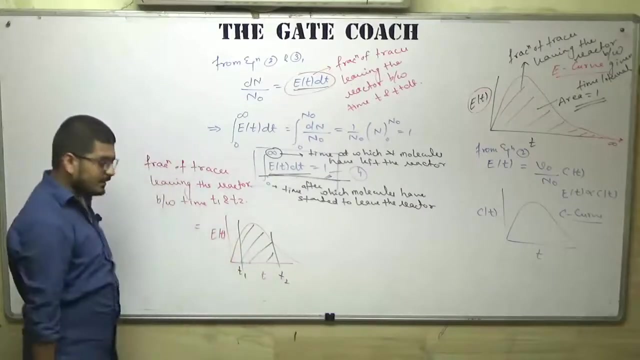 this flexible không number on belong Re. so let's find the fraction of a percentile: рубл r1, real number r1, its from R1 until t1, h1. second tracer from r opt t1. so here we will write the fraction of r with t1. 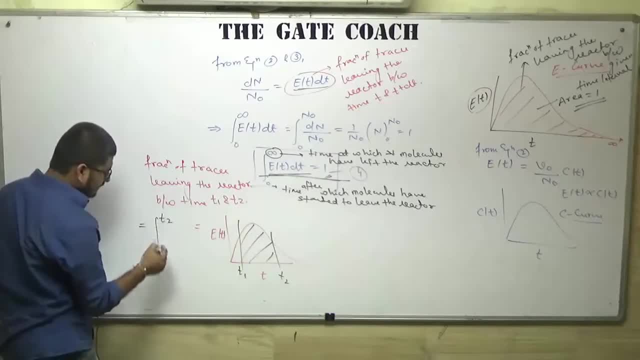 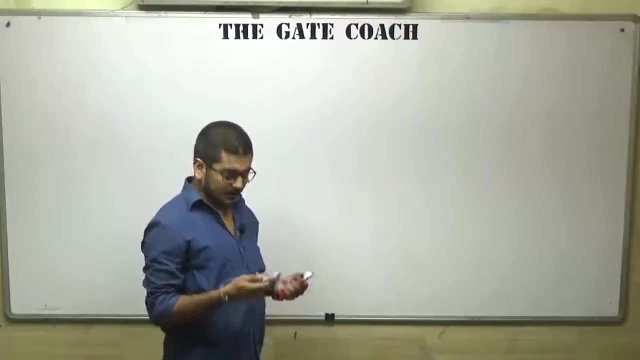 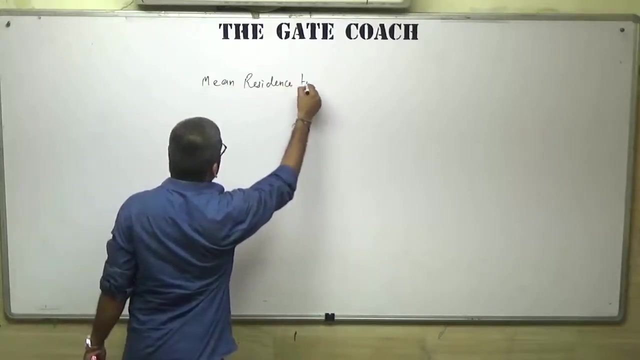 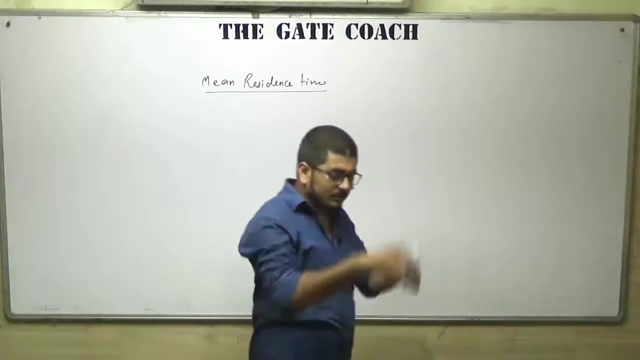 rb, t2, rb, s, t2, rb. Now there is one more thing, that what will be the mean value of the curve, or we can say the mean residence time. we have different molecules with different residence time, so what will be the mean residence time of total reactor? so we can, denoted by that value, mean? 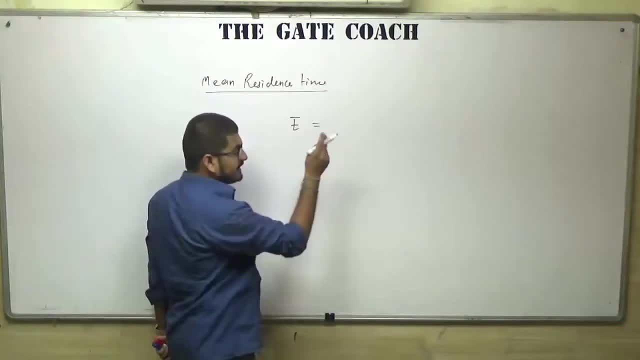 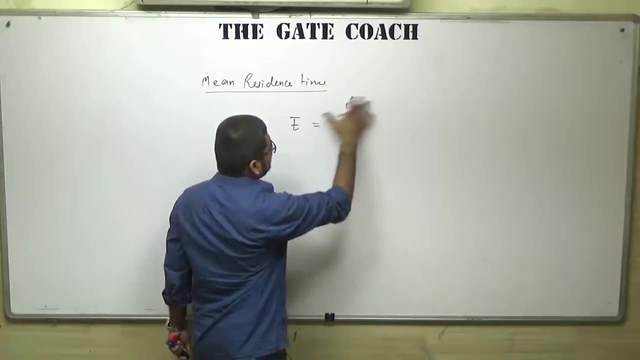 residence time by t bar. and we know that mathematically the average of any term will be based on integration, and here the distribution function is et. so based on that we can define the mean residence time. But the value of this curve, this function et dt, from 0 to infinite will be 1, so t bar. 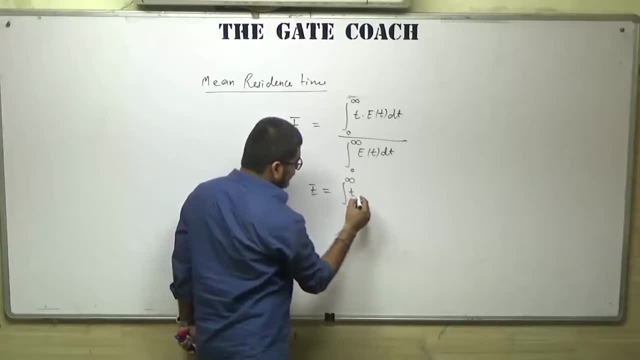 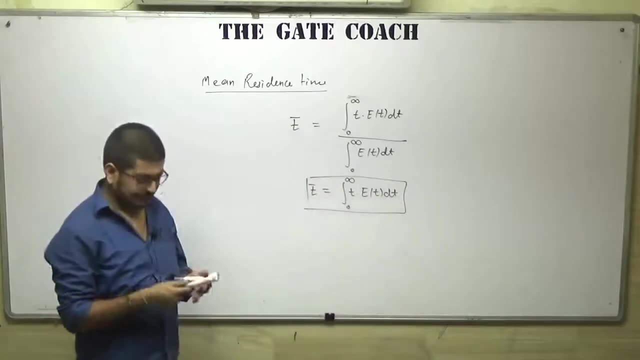 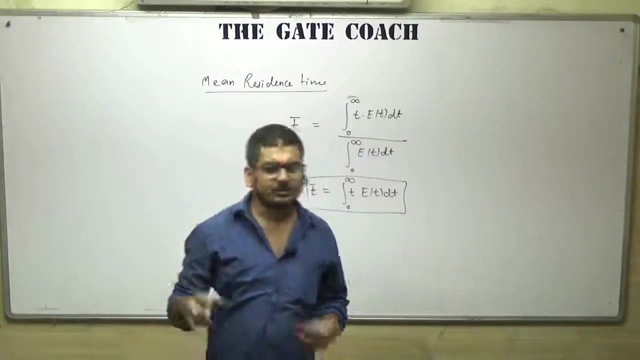 will come out to be 0 to infinite of t into et dt. and now we know that in industry we are dealing with mixture, so we define normally concentration terms. we don't deal with moles for the mixtures. So the exit from equation 1.. 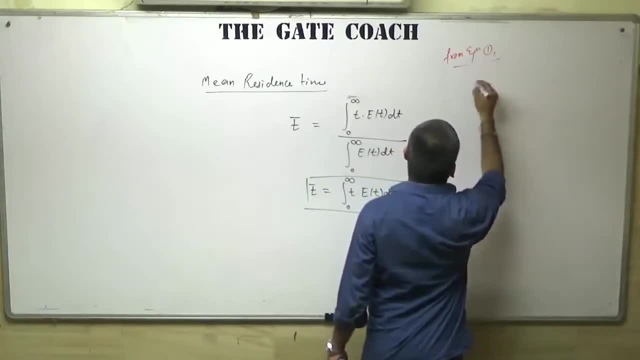 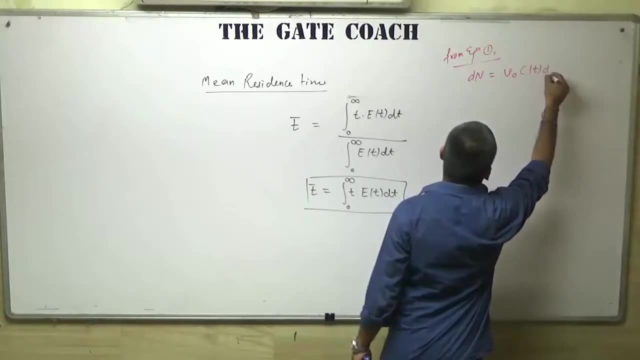 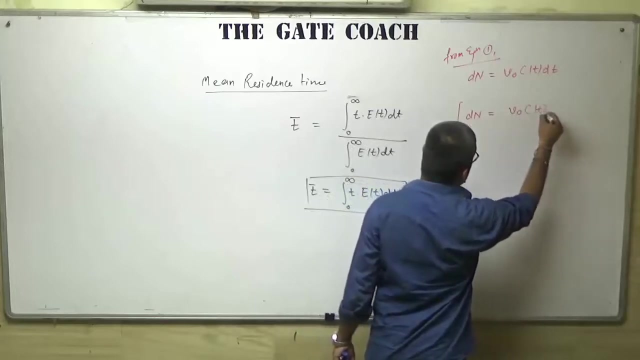 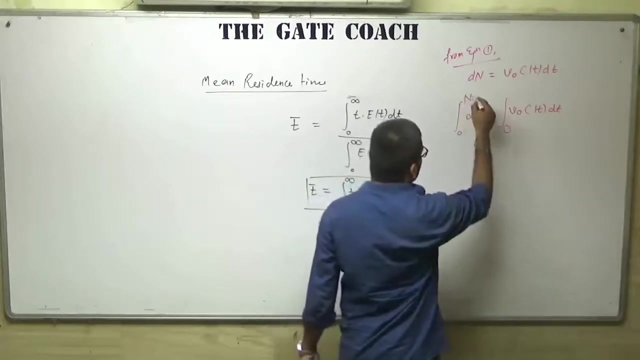 You know that we were having: dn is equal to v0, ct into dt. so if you integrate this function at time t equal to 0, molecules leaving the reactor will be 0 and time required by the molecules, all molecules- to leave the reactor will be infinite. 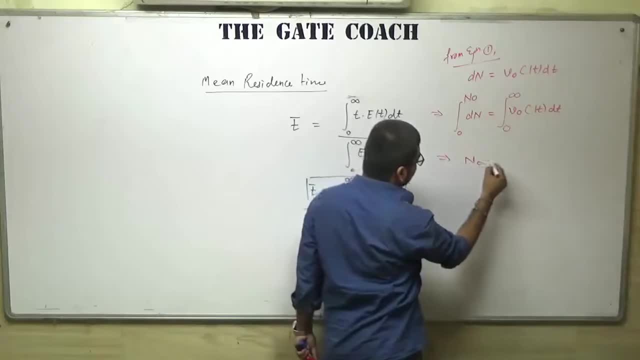 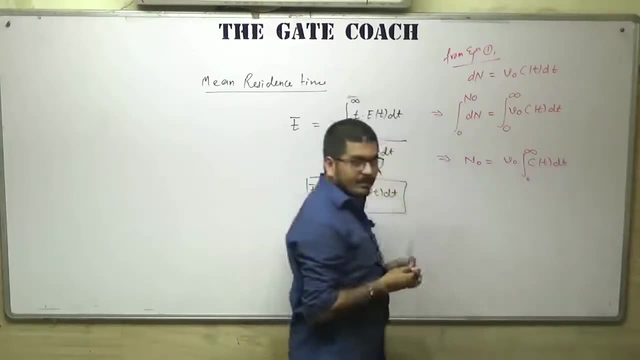 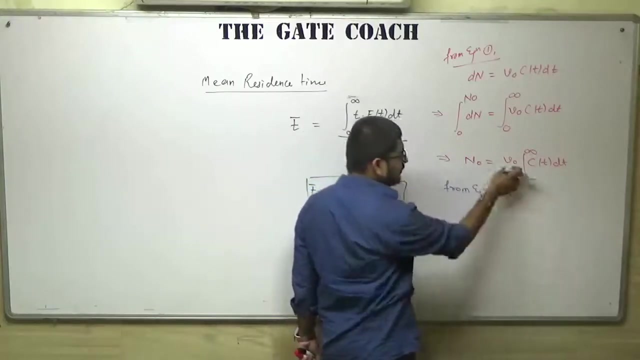 Okay, Okay, So it will be like: n0 is equal to v0, integration from 0 to infinite, ct into dt. and now from equation 3, if you know that n0 over v0 can be written as: ct over et is equal to 0 to. 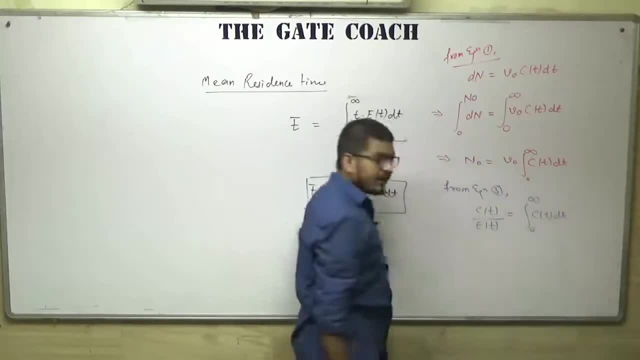 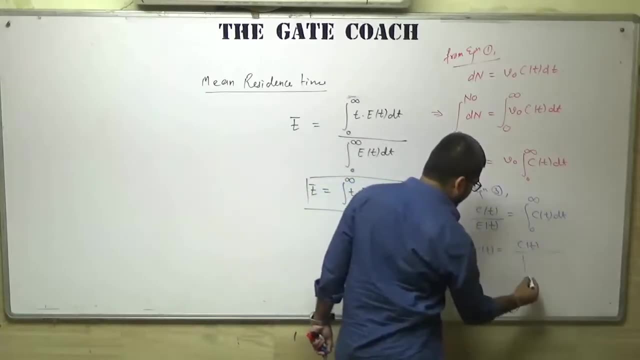 infinite integration of ct, dt. Okay, So the et will come out to be like: Okay, Okay, So now you write me Right Now you have 1 over 1, something which is equal to the second integral ct, dt, plus integration from 0 to infinite of ct to dt. right, any question, 5, 6, whatever. it is okay to now see. 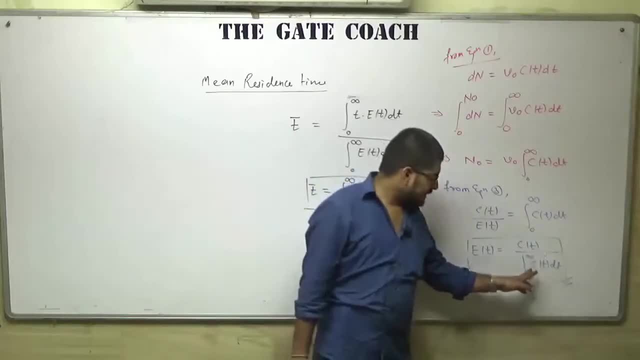 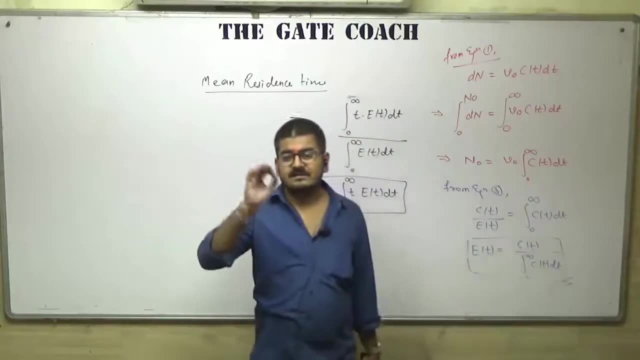 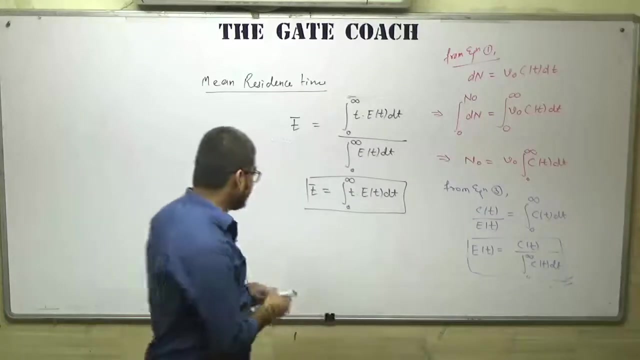 et is equal to ct over this. and what is this part denominator integration is of ct, dt, from 0 to infinite. and what is ct? ct is the concentration of tracer at exit of the reactor. Means it is a result, means it is a result, and this is basically the area of C curve. now tell: 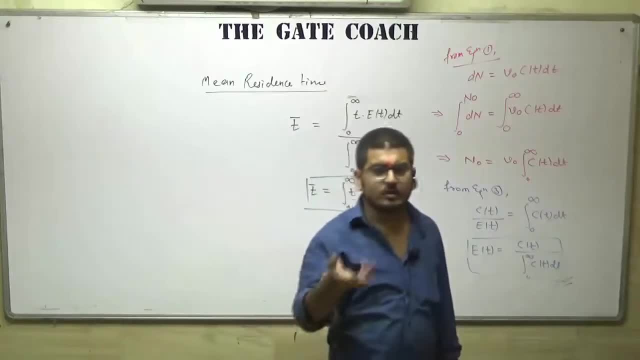 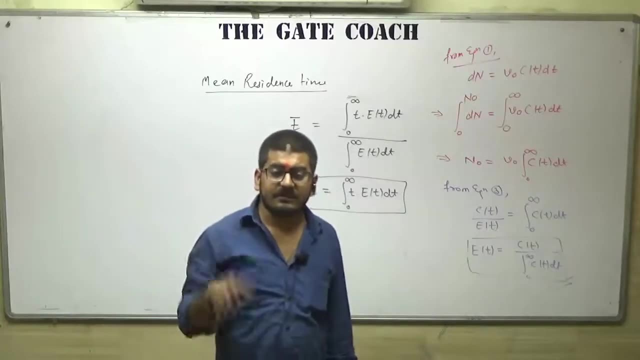 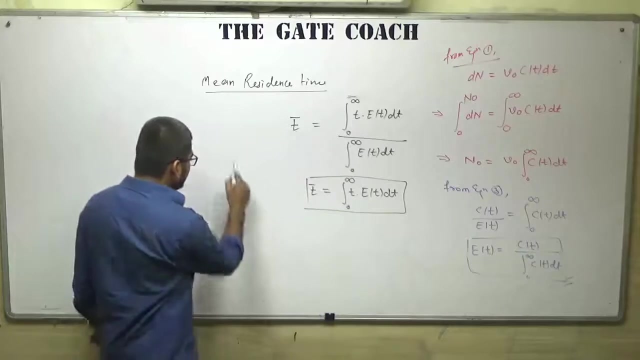 me one thing: all of you have must have cleared your 12th and 10th examination. so can you change your 10th result, the value of 12th result? no, obviously, because those are results and those are constants. so, in the same way, in C curve, which is the curve between exit, concentration of tracer, 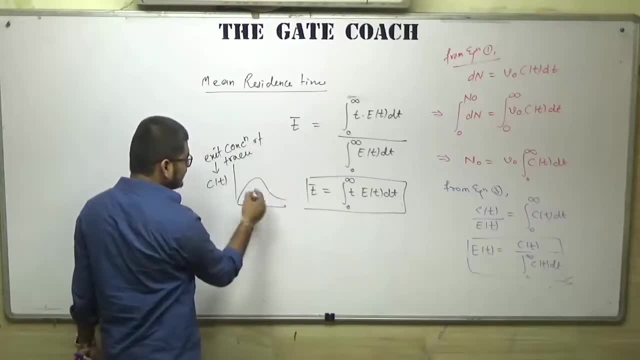 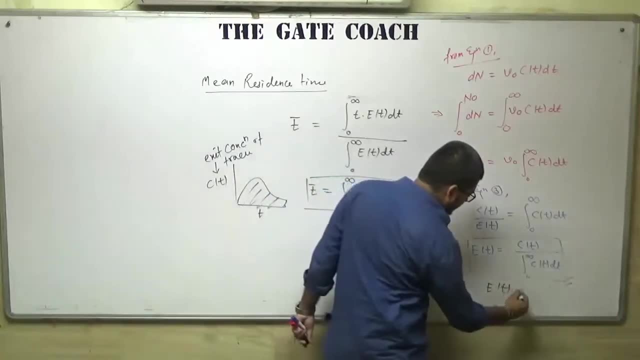 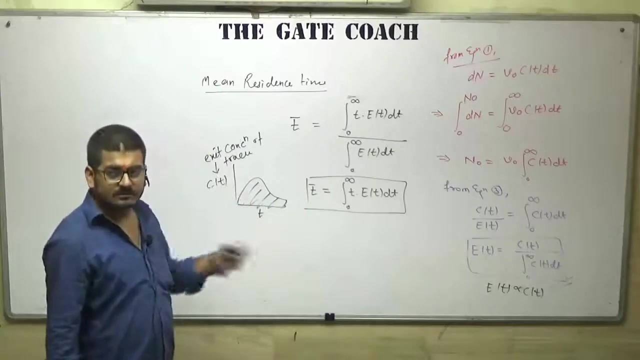 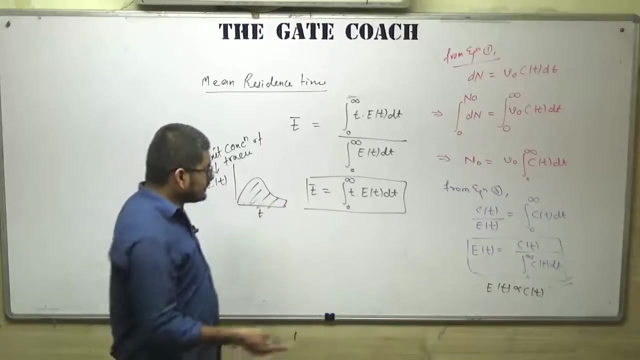 versus residence time, which is a result. so this area will be constant. so, ultimately, ETE is proportional to CTE, because this is constant. so that is the area of C curve and C curve is the result, outcome of the process. so the values will not change after coming out. So now, when you put that value in this equation, you 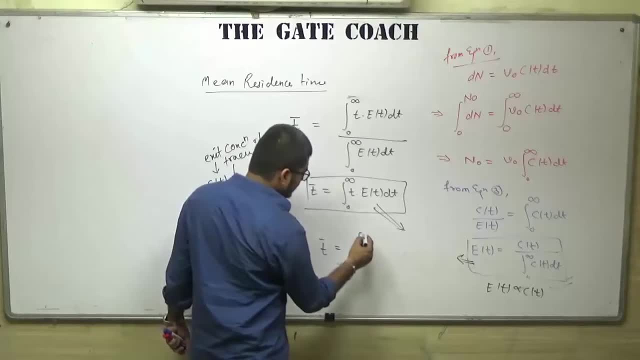 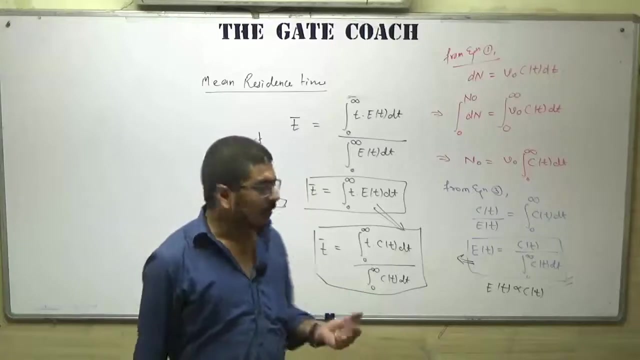 will get. t bar is equal to integration from 0 to infinite of t into ct. dt divided by integration from 0 to infinite of ct into dt. So this is one way to find out the mean residence time. So this is something about pulse input experiment and all. There are so many points. 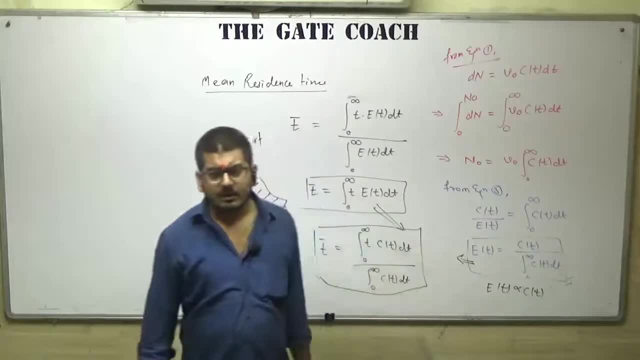 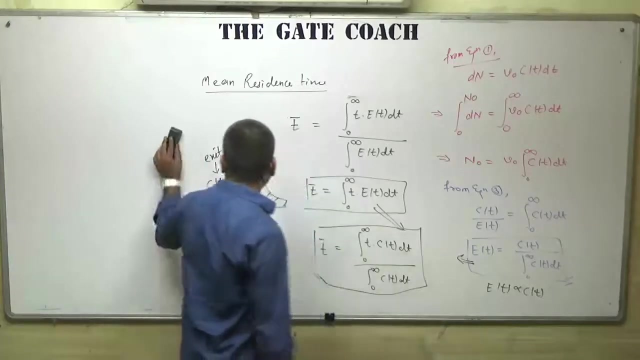 to discuss that. we will discuss in class. If you have any doubt, then you can ask that in your comment section. Now I am just wrapping all this by solving our numerical from the gate Examination, which came in the gate exam from 2005 or 2006.. So there was a question in. 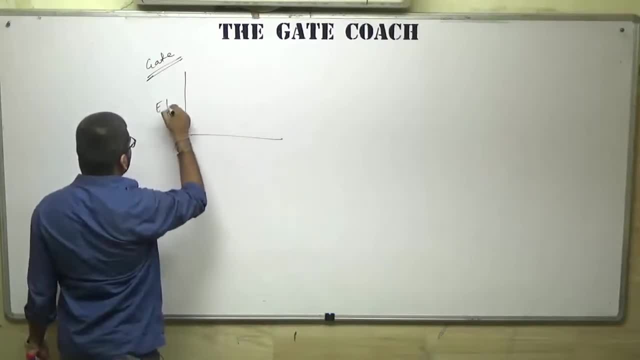 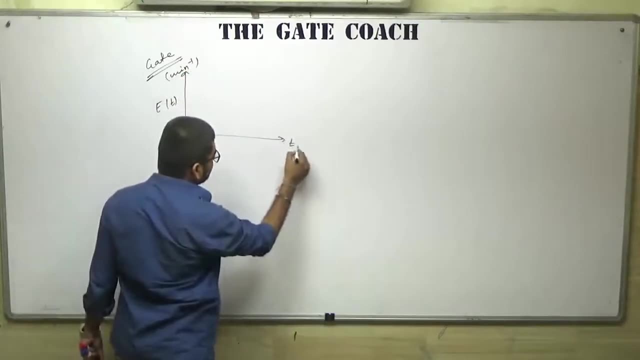 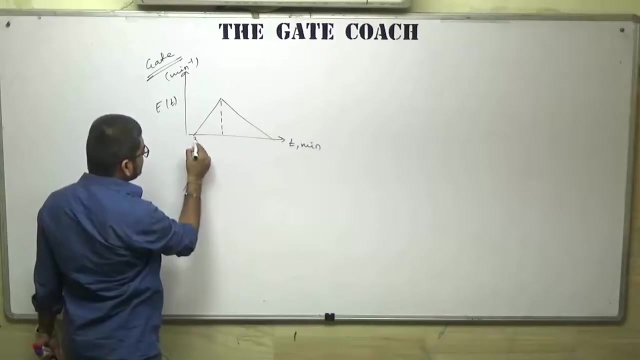 gate exam that we have given our E curve. The units of exit age function is minute inverse versus time, that is, in minutes. The curve is something like this: This is 3,, 8,, 15,, 0, 0 and this value was E max. So I asked you first, what is the value of E max? and second, 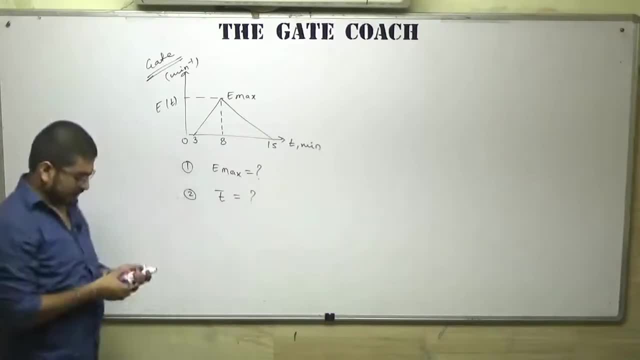 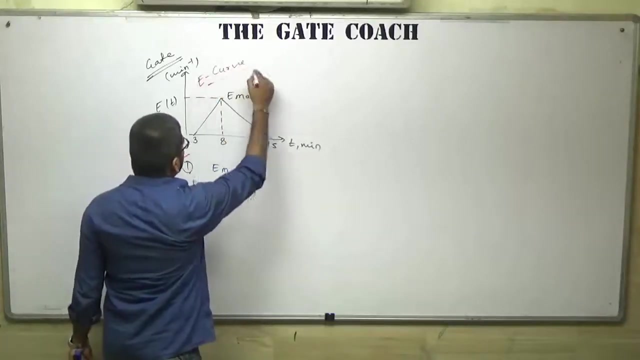 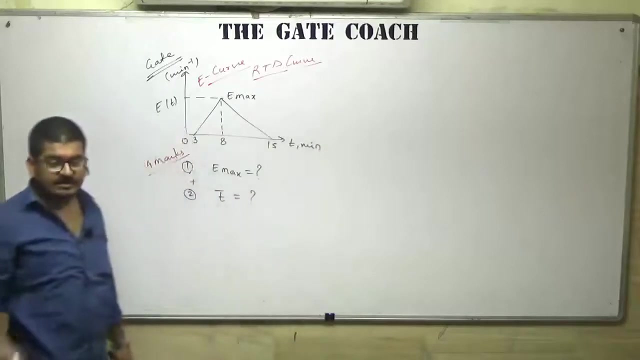 what is the value of mean residence time? So this question was there for 4 marks, 2 plus 2, sorry. So it is a very simple question. for a pulse input experiment, RTD curve was was given. this E curve is basically known as RTD curve of the reactor. remember this. 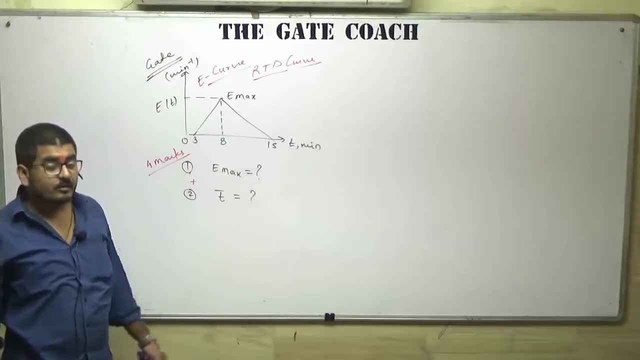 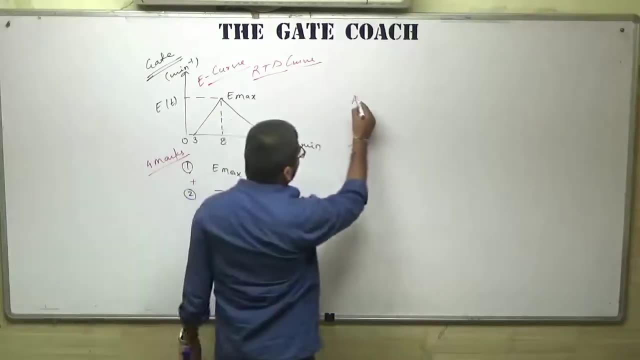 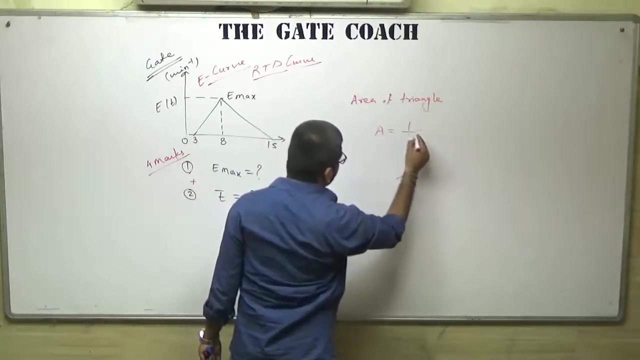 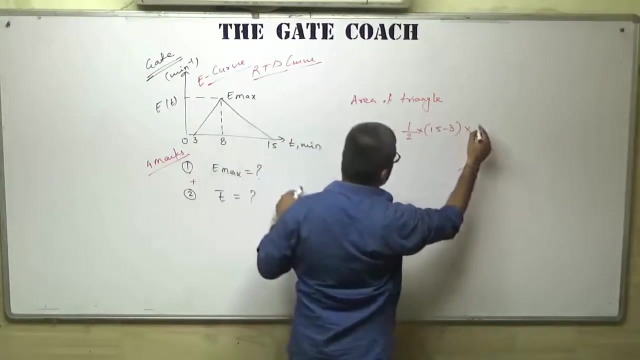 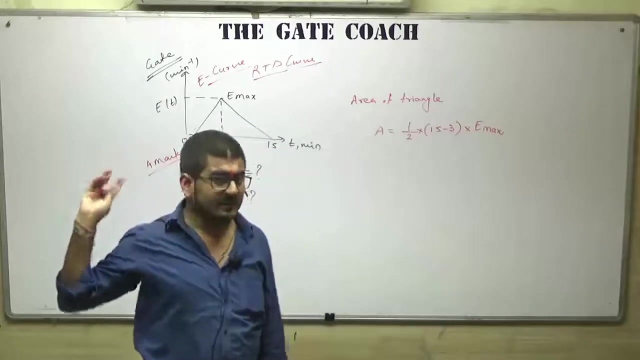 So now you have to calculate E max, and we do not know how to calculate that, but we can say it is a triangle and we know that area of a triangle can be written, calculated by half into base, into height. Okay, and because form the definition of E curve? we just calculated that the area of 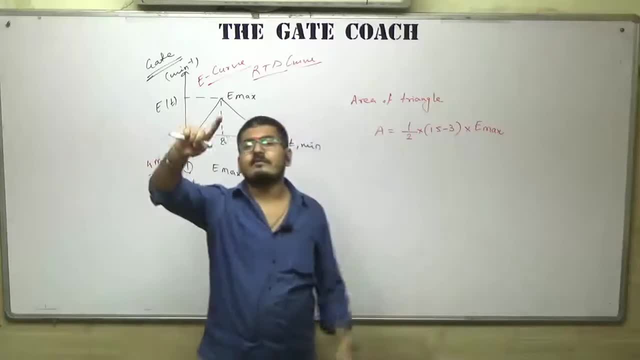 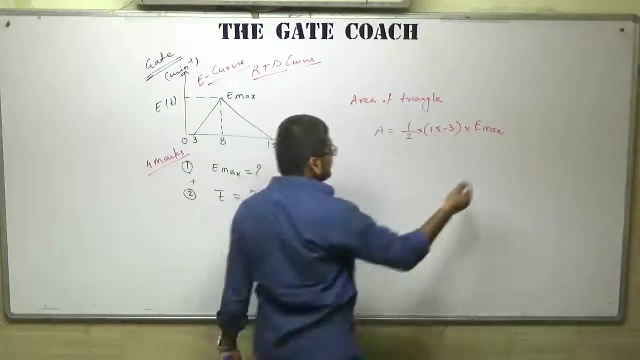 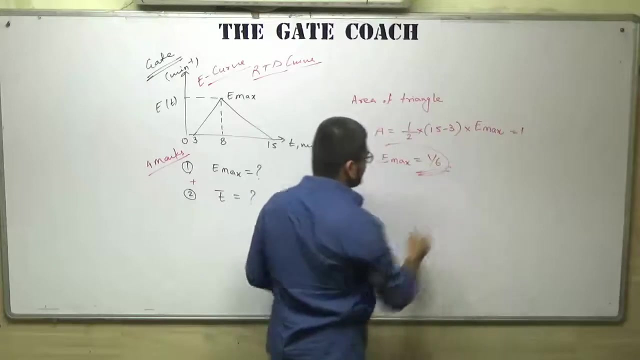 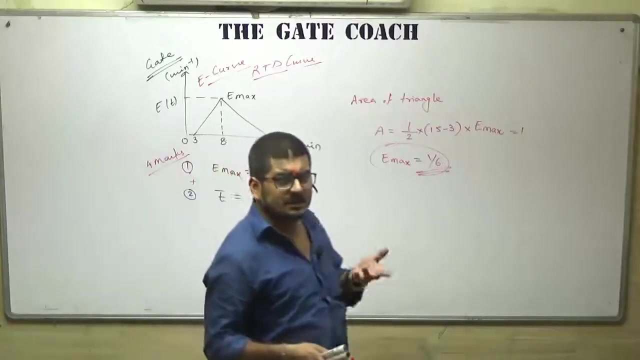 E curve in the total interval will be 1 always. so here, in the total interval from 3 to 15, the area of E curve will be 1, so the value of Emax will be 1 by 6. very simple. this question was there for 2 marks. okay, you can imagine which kind of questions are. came in exam, okay, 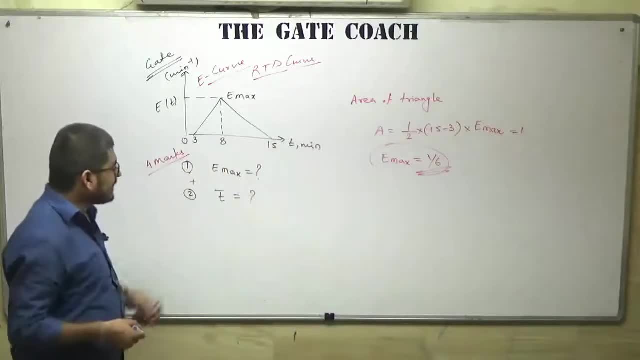 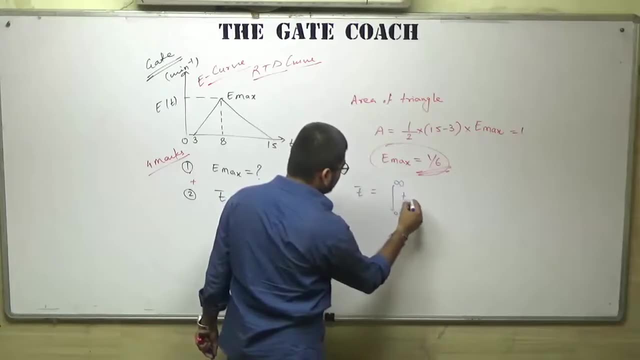 very basic conceptual question. next, is T bar mean residence time. so we know that T bar can be calculated by the equation like this: okay, so for this curve the equation will become: will become: the time after which molecules started to leave the reactor is 3, the time 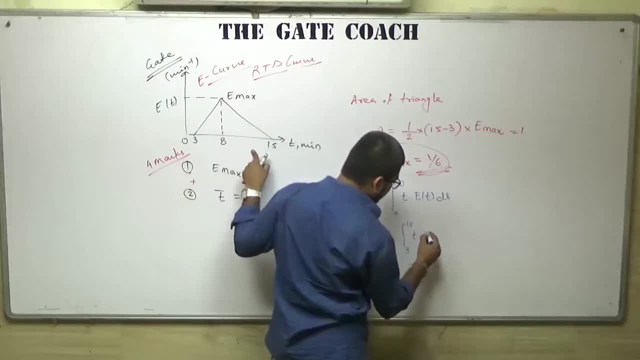 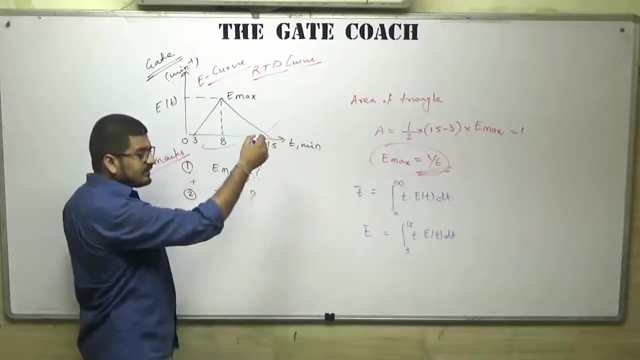 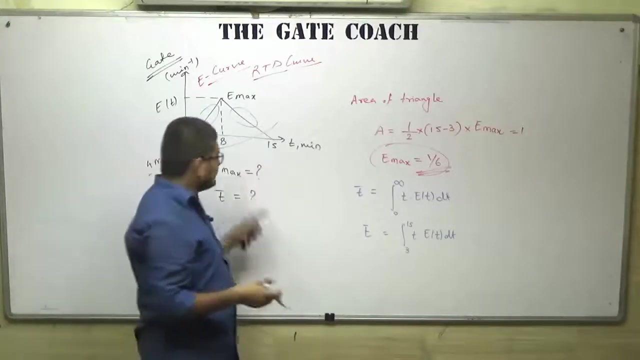 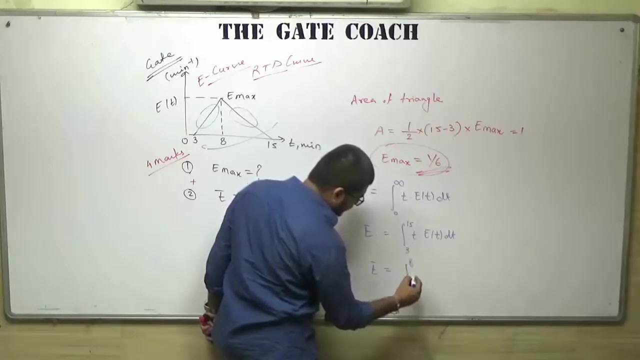 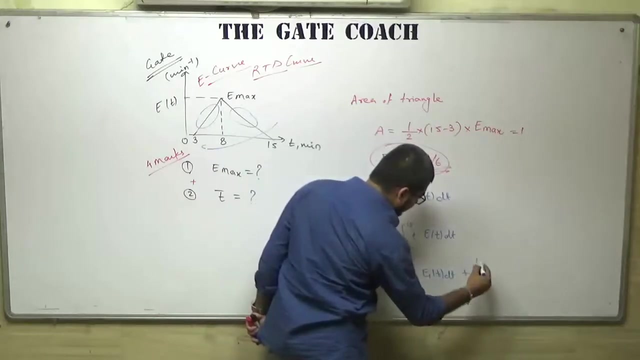 till which molecule left the reactor. 15 T into Et DT. Okay, but now we can see in this function, in this curve, there are 2 slopes. curve is changing, okay, slopes are changing between the time intervals. so this T bar can be written as integration from 3 to 8 of T into E1, T DT, plus integration from 8 to 15 of T into E2. 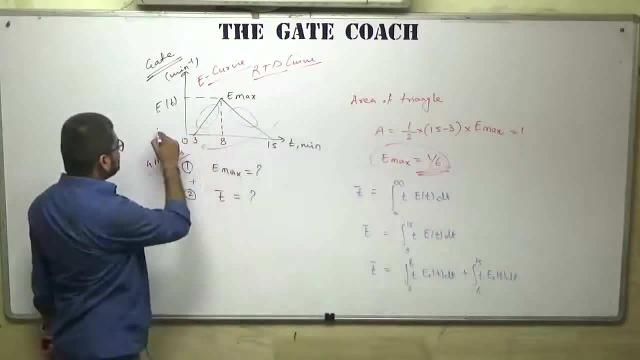 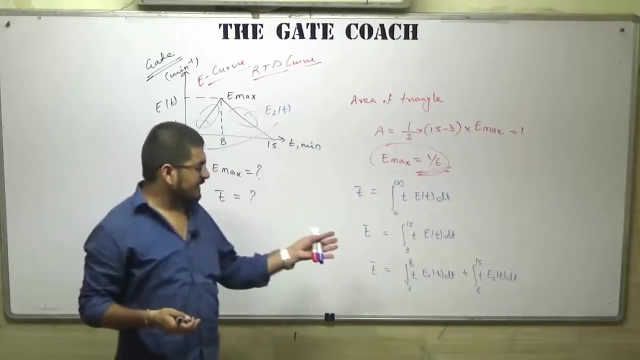 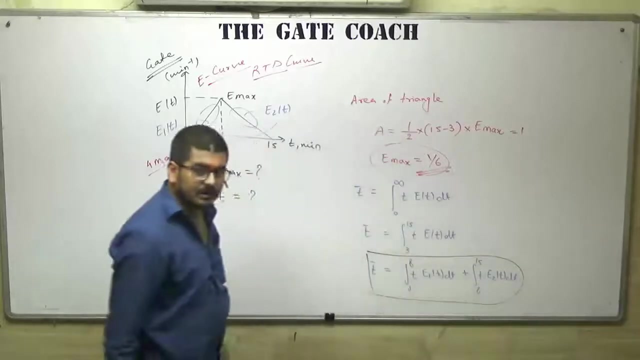 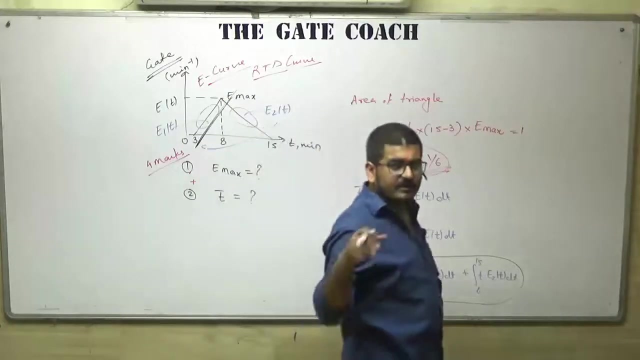 T, DT. let's say this part is E1 and this part is E2T. okay, put the values of E1 and E2 as a function of time in this equation and you will get your answer. okay, now how to find out C. this is what a straight line equation and we straight line curve and we know that. 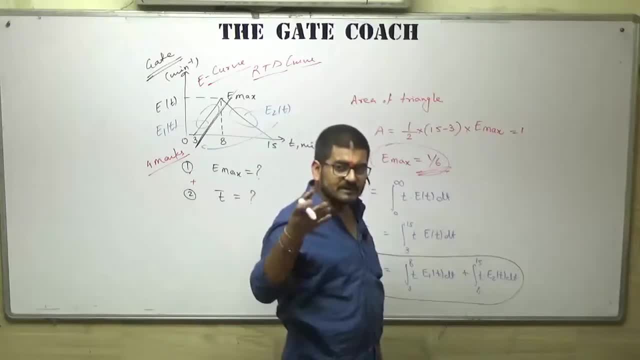 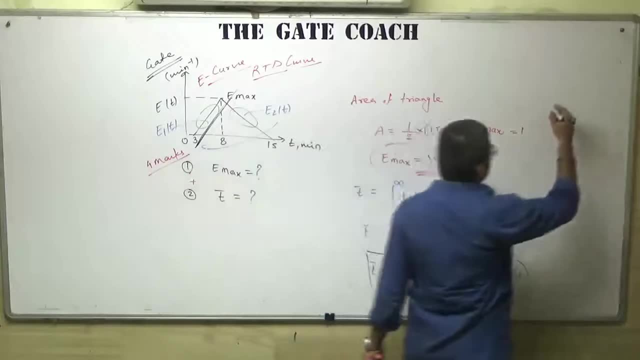 the equation used to represent the curve is E2T. Okay, Okay, Okay, So straight line curve connecting between 2 points will be like: Y minus Y1 is equal to Y2 minus Y1 over X2 minus X1 multiplied by X minus X1. okay, so for this case it will. 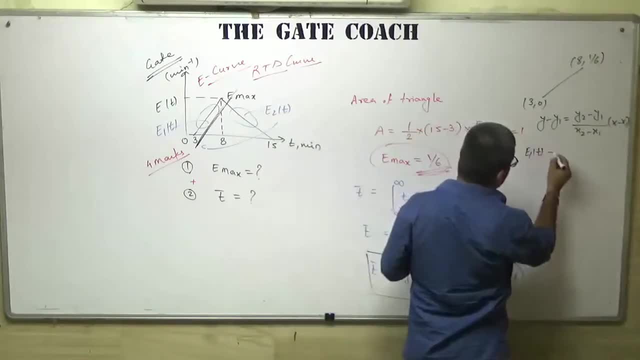 be like: on Y axis we have E, E1T minus Y1, that is 0,. Y2 minus Y1, that is 1 by 6 minus 1.. Okay, X2 minus X1, that is 8 minus 0,. X2 minus X1, that is 8 minus 3. on X axis we have T, so it 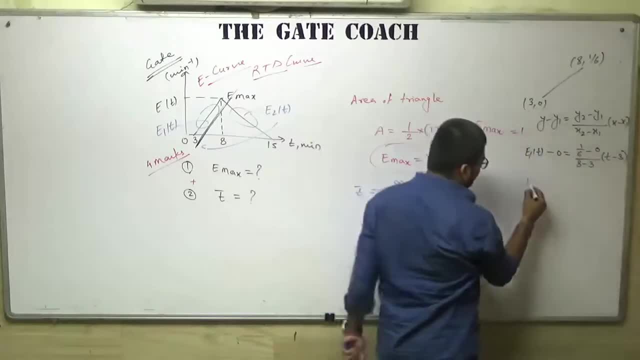 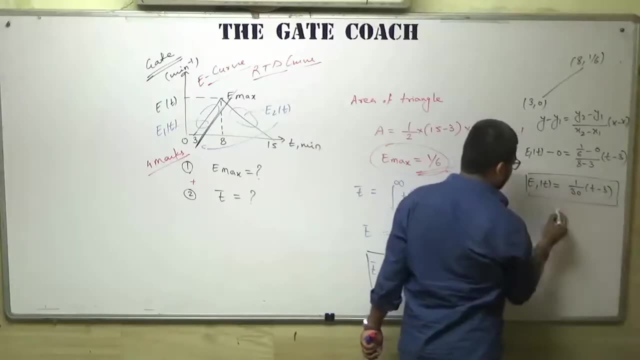 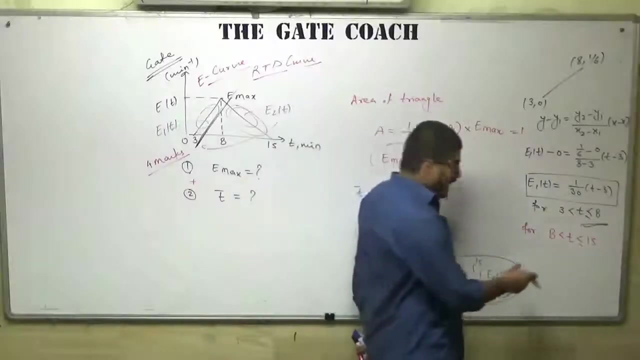 will be T minus X1, that is 3, so here you will get. E1T is equal to 1 over 30 T minus 3, and which is valid for time between 3 to 8, okay, and for time between 8 to the function of. 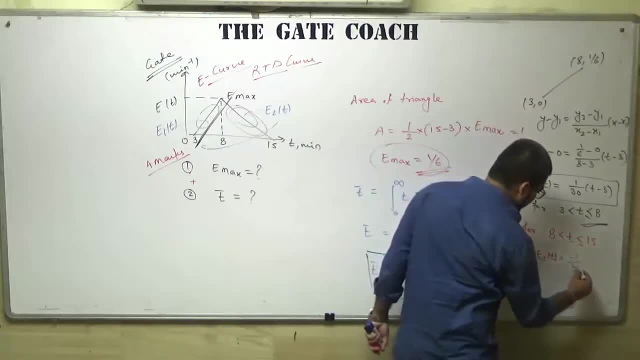 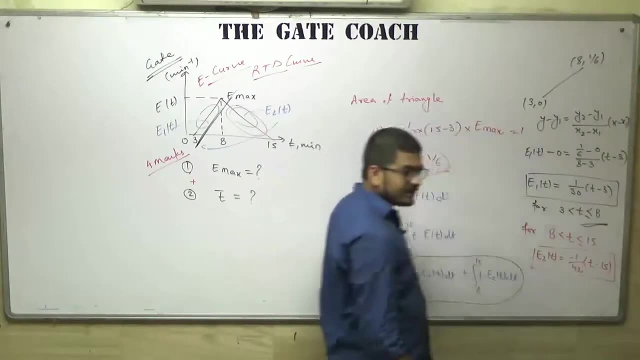 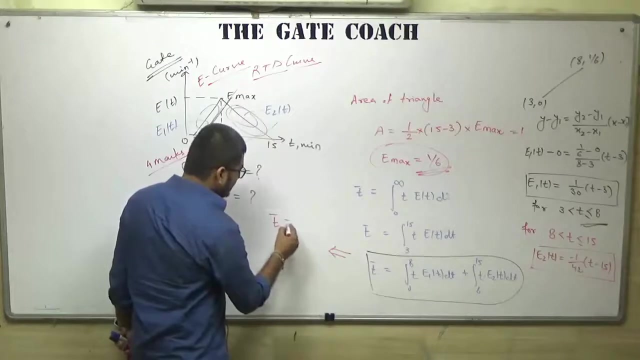 E2 will come out. Okay. Okay, Now you will get minus 1 by 42, T minus 15, which will be valid only for this time interval, and when you put all those value of E1 and E2 in this equation, you will get T. bar is: 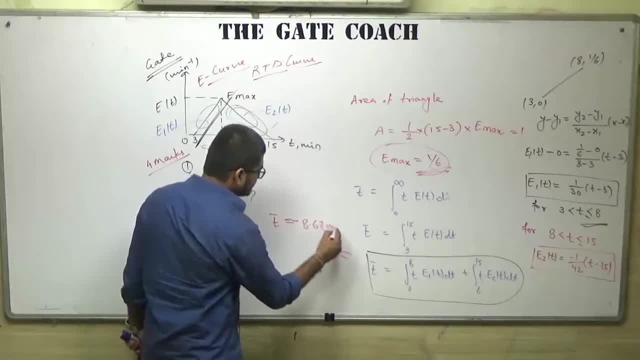 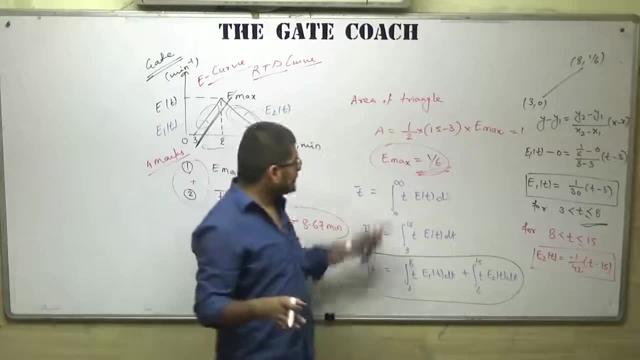 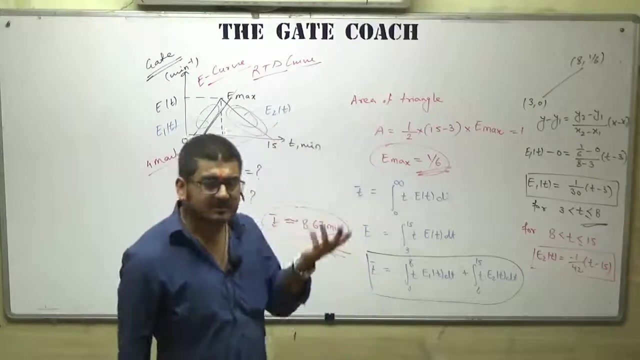 equal to approximately 8.67 minutes. Okay, And this question was there for 4 marks. very basic question. you just need to put the values in the equation. Okay, know the equation, you can solve it, but the meaning of the terms should be clear that. 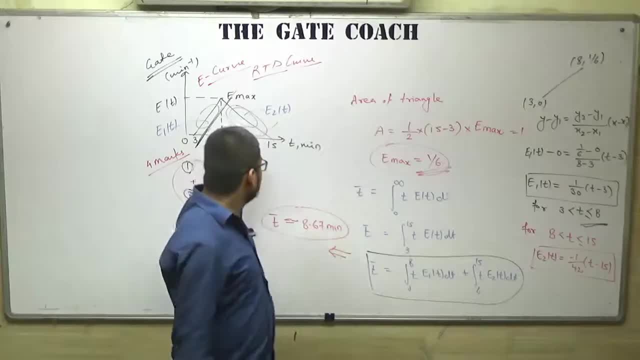 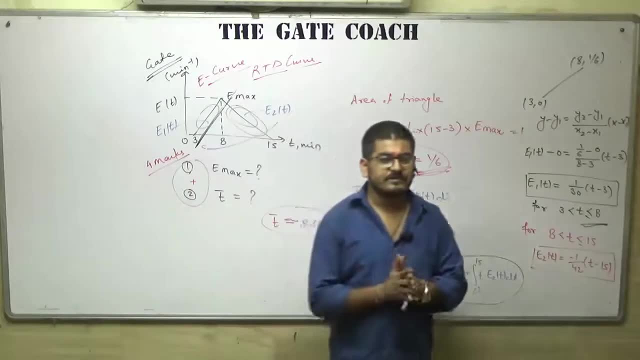 the area of E curve will always be one between total time interval, the T bar, E max and also all those things. So this is all about the pulse input experiment which I want to discuss. there are some more part in RTT chapter that we will we cannot discuss obviously here in.